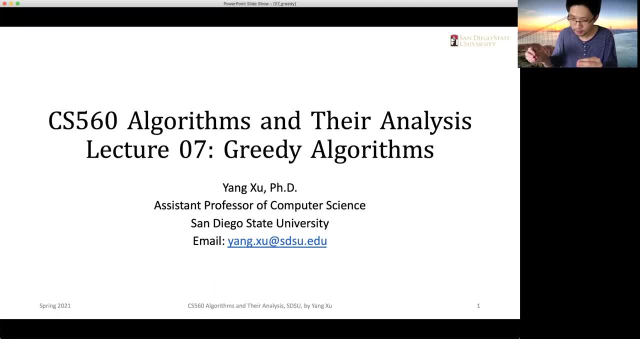 Okay So, the optimal structure is that we need to solve the right part. the remainder parts use the same algorithm. Right, We want to know the optimal revenue for the right part. Okay So, and in order to obtain the optimal solution for the original problem, 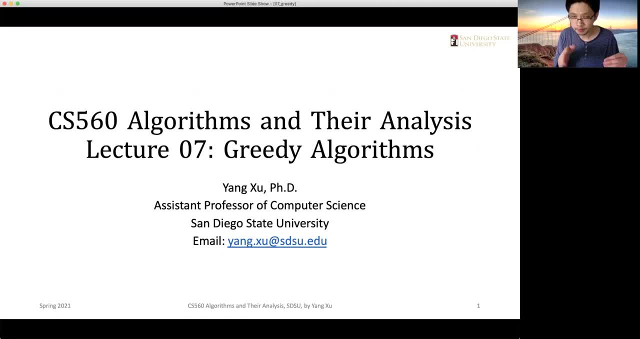 we need to explore all possible sub problems. We need to solve all possible sub problems, And that is a characteristic of dynamic programming approaches. Right, We need to explore the sub problem space exhaustively. We need to. we don't want to miss any. 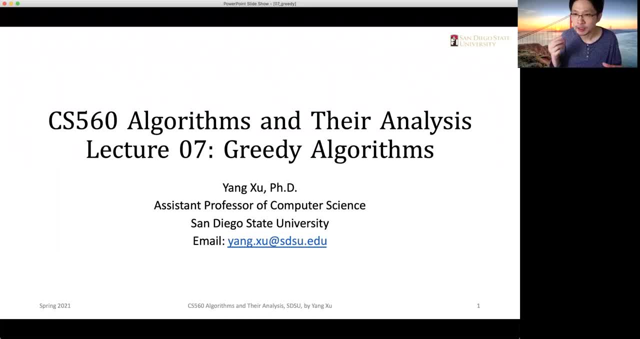 possible sub problems, Because our goal is to have the optimal solutions. That means we need to compare all possible solutions, Okay, So that's why dynamic programming requires some some good top-down. I mean top-down design like top-down math, overall design of the. 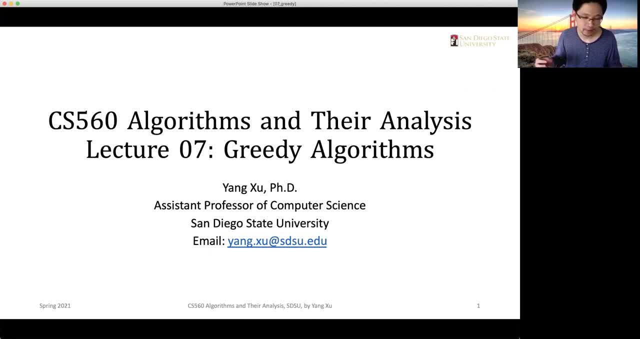 of the, an overall idea of how many possible sub problems are out there. Okay So, which makes it a a difficult approach, or well, not that easy approach to understand. Okay, So let's back to go back to the topic this week. 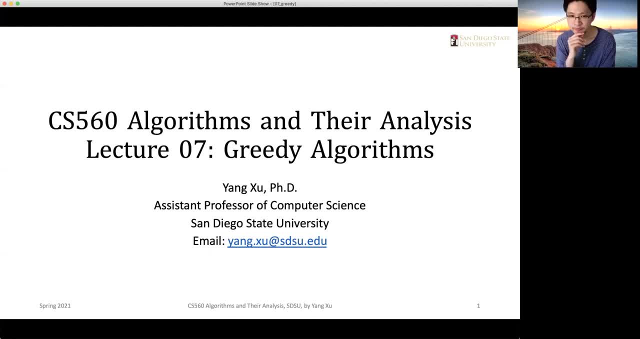 The greedy algorithms is a type of algorithm that can basically solve problems in a similar way to dynamic programming, Like we need to get the optimal solution to some problem- Okay, But the good news is that in the greedy algorithms we don't actually need to. 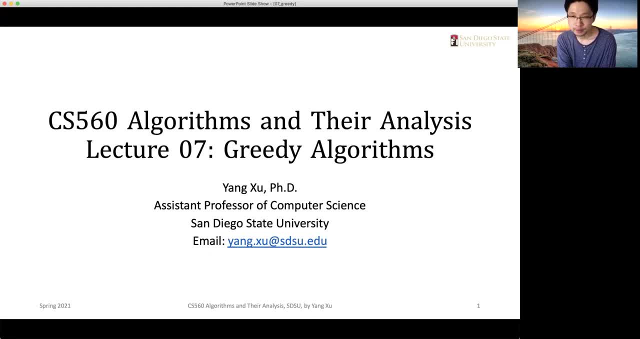 exhaustively exam all possible solutions. Okay, We will need to use some heuristics to choose to make the locally optimal best, the locally optimal solution, rather than making sure that our current local solution is the global best solution. Okay, So which saves us time to. 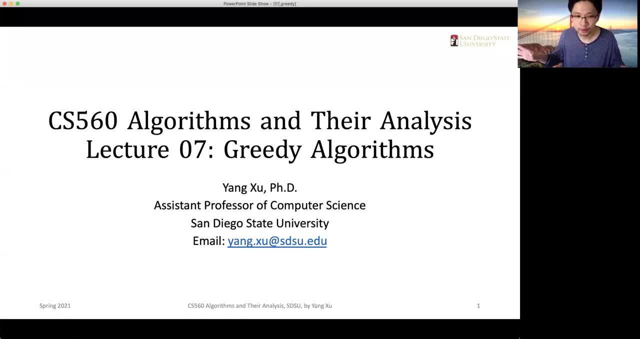 look to, to look at more, more sub-problem space To a bigger sub-problem space. Okay, So it. in terms of results, in terms of running time, the greedy algorithms is usually a pretty efficient algorithm compared to dynamic programming algorithm solutions. 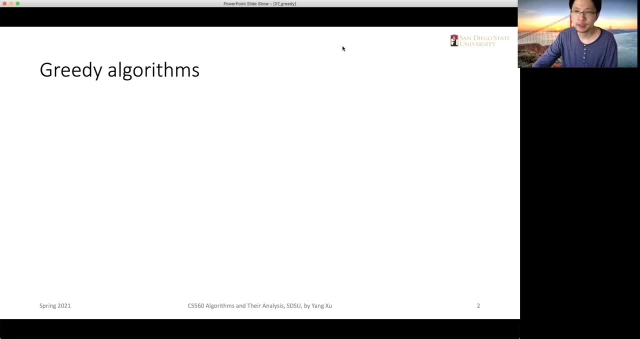 Okay. So I think it will be easier to understand it if we go through some concrete examples, And in this chapter we will basically cover three concrete examples. The first one is called activity selection problem, And then we will cover Huffman codes And lastly, 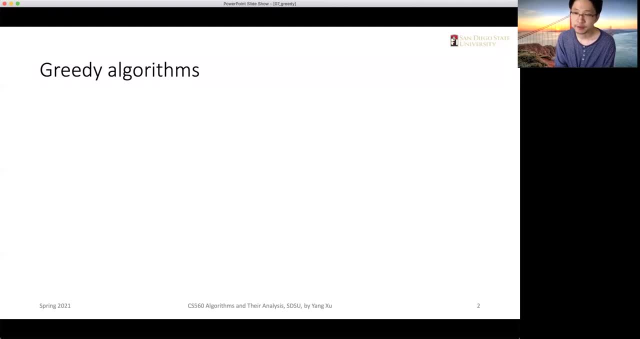 we will spend some time on a very classical example that connects greedy algorithms with dynamic programming. Okay, We will see how the same problem can actually be converted to a dynamic programming problem. And then, how did it really? how it is related to the 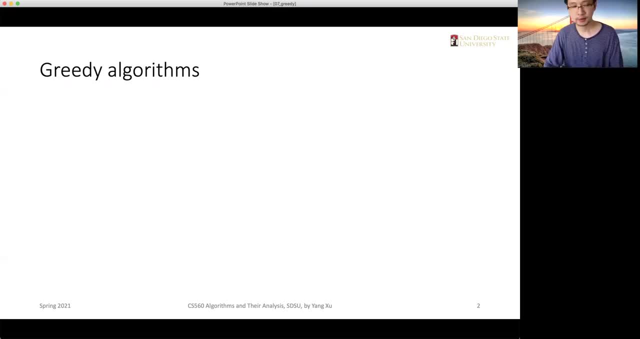 to the greedy algorithms problems. Okay, All right, But still some theoretical discussion would be helpful at the beginning. So greedy algorithms: it's it's usually suitable for optimization problems, which means we need to go through a sequence of steps. Okay, 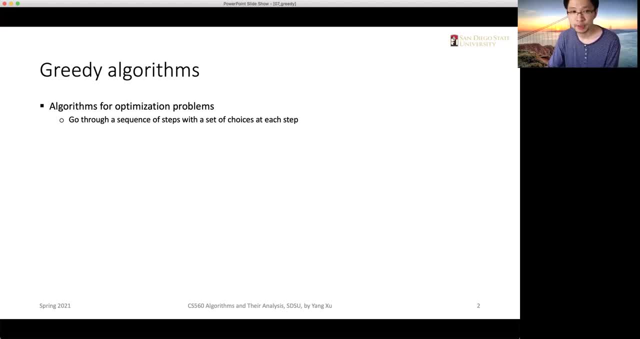 And at each step we need to make make a choice about several options. Okay, So generally speaking, the general principle of a greedy algorithm is that whenever we need to make a choice, we always make the choice that looks the best at the moment. 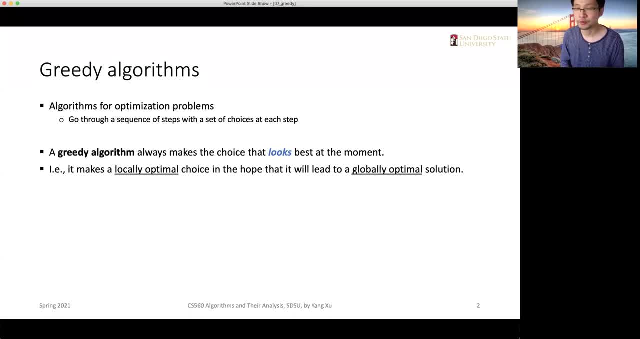 Okay, By it looks the best, we mean that we just make a choice that looks like some locally optimal choice. Okay, Without the global information. Okay, We are not sure whether our current choice will actually lead to the global, globally optimal solution. 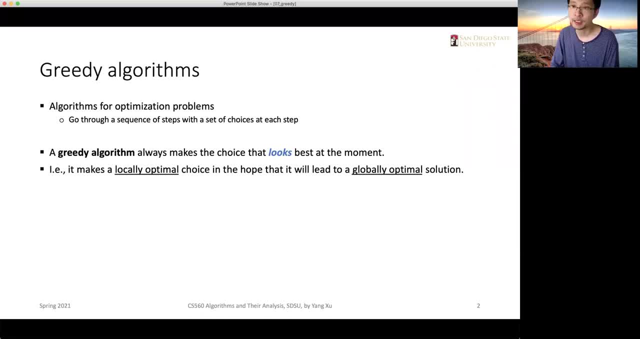 Okay, Of course, this is risky, because sometimes the locally best choices is not necessarily the globally optimal one. Okay, So it depends. So how? whether the greedy algorithm can apply to certain problems actually depends on the nature of the problem. In some cases, 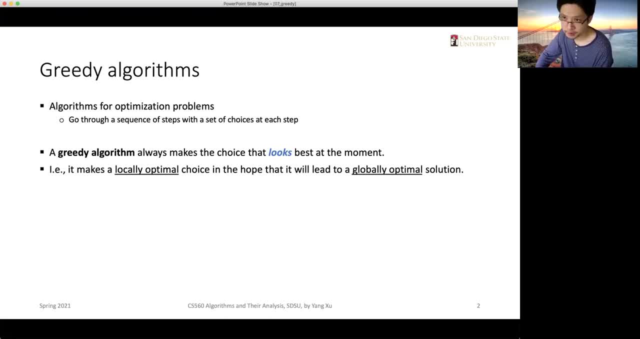 the greedy algorithm is not sufficient to solve the problem, but sometimes it's just okay. Okay, And in those cases where greedy algorithms works, usually speaking, the same problem can also be solved by a dynamic program. Okay, But in those cases? 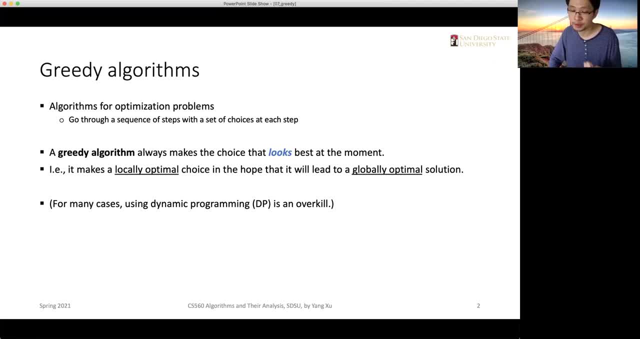 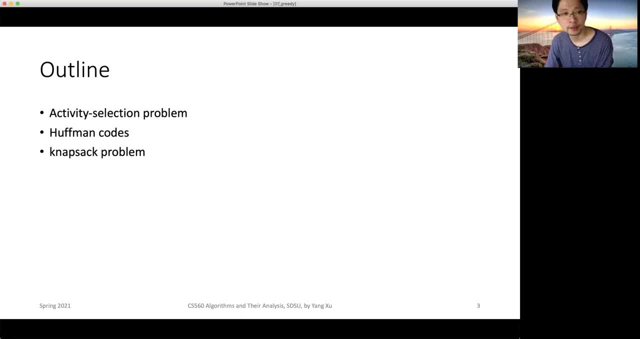 dynamic programming is just an overkill. Okay, We don't necessarily need to fully explore the subproblem space. All right, So, as we said, we will look at three specific problems. So today we're going to cover activity selection problem. 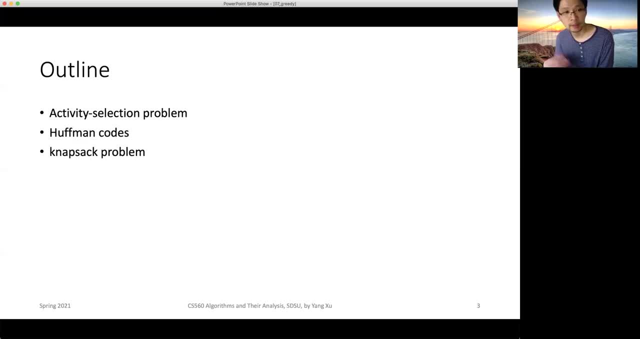 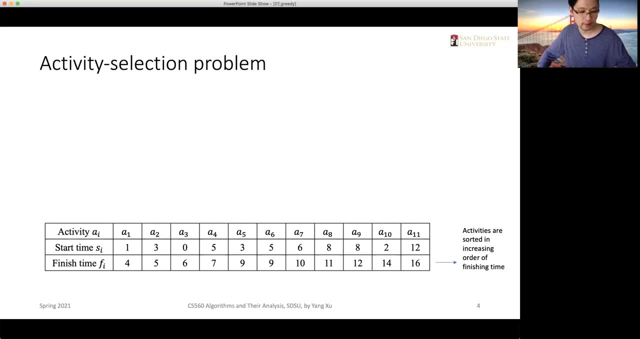 And then on Thursday we're going to cover Huffman codes and maybe with Knapsack problem as well. Okay, All right. So let's look at this very practical problem. We actually come into this type of problems in our everyday life. 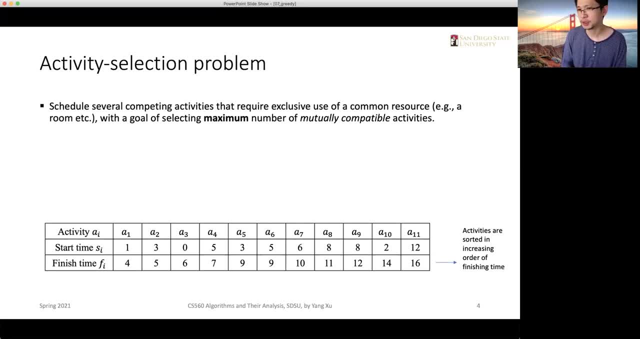 Okay. So it's about scheduling. Okay Say, we have a, we have some resource, We have a room space right which is vacant And we want to like schedule a lot of activities. okay, using that room. 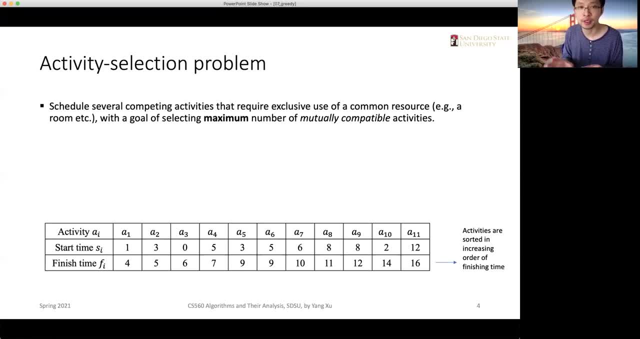 Okay, And those activities actually compete with each other, right? We, only we, we, we, we need to know that, we need to make sure that there's no conflict between between those activities being scheduled right, Because they exclusive. 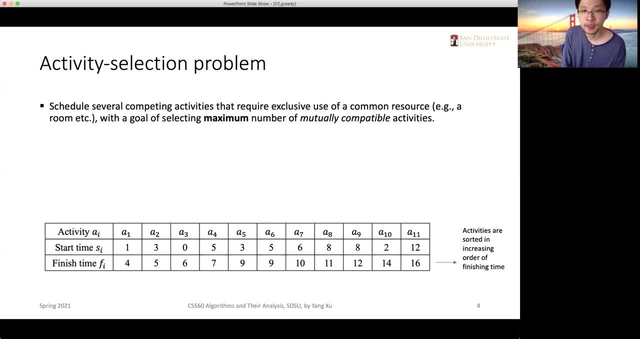 they require exclusive use of the same room. Okay, So if I'm a manager of this room, right? So the goal for me is simply to select, to to schedule as many prob as as many activities as possible, right? 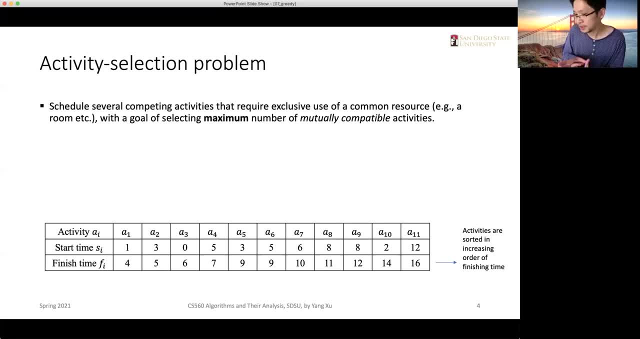 As long as they are mutually compatible, as long as the the first activity does not conflict with the second one, the second one doesn't conflict with the with the third one, right? So so that I'm making the most out of this room. 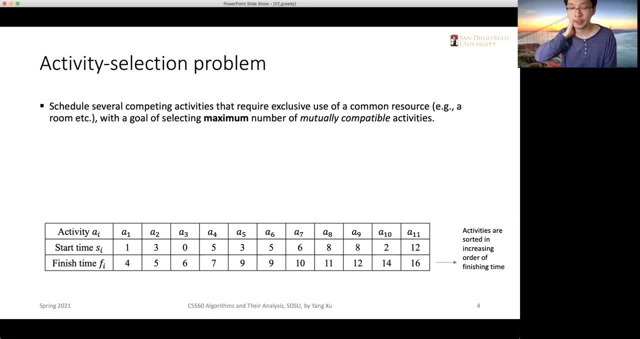 right. So this is a a very typical situation where we have some goal, we have some goal, we have some resource and we want to optimize the, optimize the outcome based on our selection. All right, let's further lay out some conditions. 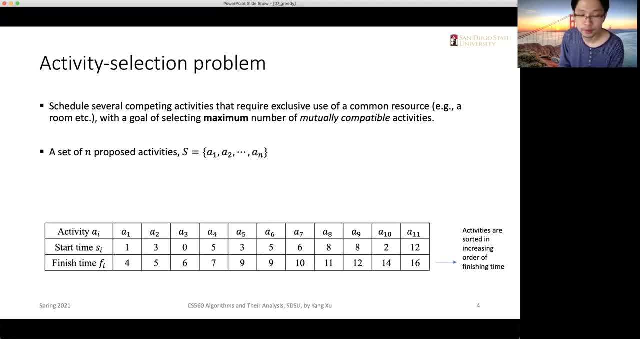 Say, we use the notation A1 to AN to represent the activities being proposed, Okay, And also we need, we need to have the information of the start time and the finish time for these activities right, So that makes sense. 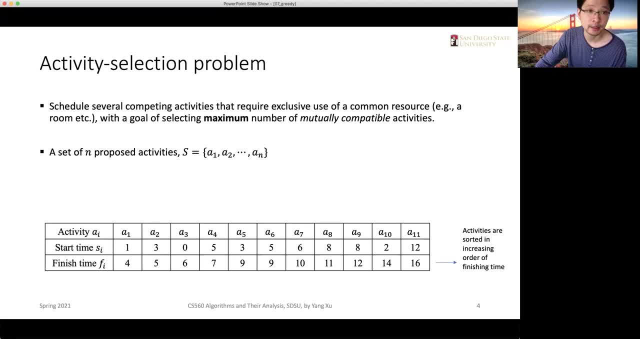 right In order to we. we have full information about the candidate's events, candidate's activities. Okay, And so assume that the start time and finish time for each activity is listed in this table. We have three rows right. 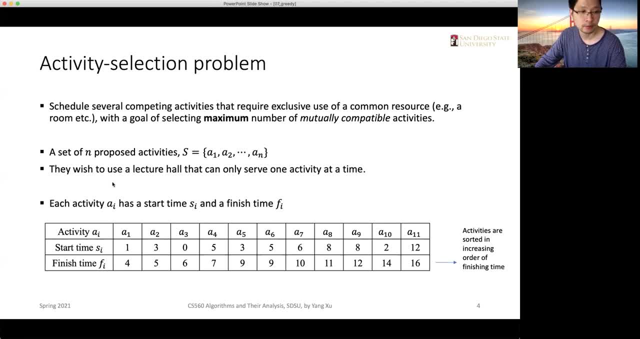 The second row is the start time right, Start time. We use SI to indicate start time and FI to indicate finish time. The I is just the index for the activity AI. Okay So. so in this table we have first ordered. 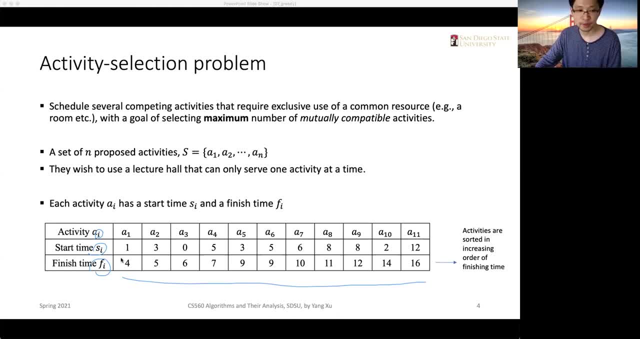 we have first sorted all the activities, So it's, it's in order by the finishing time. Okay, So of course we can also sort the activities by the starting time, but this will lead to a different kind of solution. 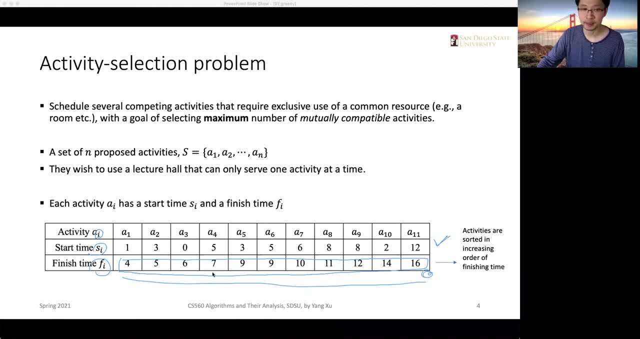 right, We will stick with this sorting by finishing time. Okay. So you see that's A1 finished by before four o'clock, A2 finished by before five o'clock and A3 is before six o'clock. Okay So. 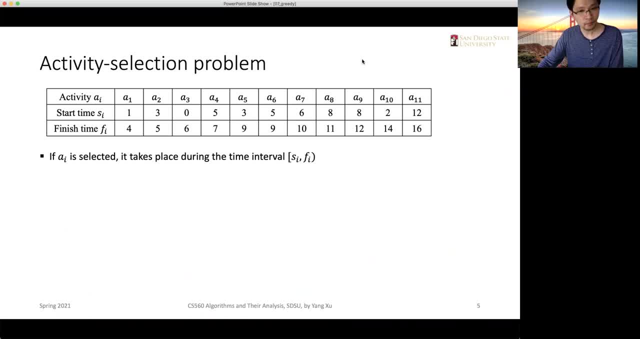 let's further observe the activities. Okay Then, if A I, the activity A I, is selected, then it takes place during time interval, like between S? I and F I. Okay, So this is the starting time. 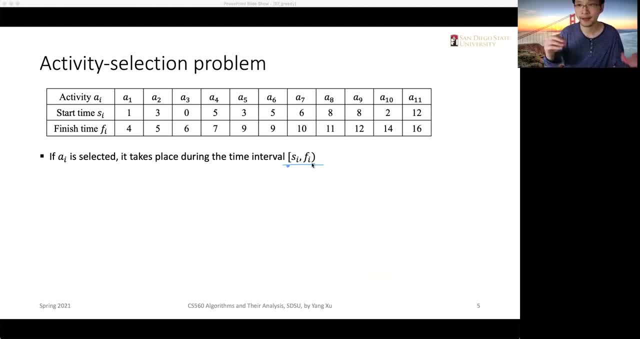 and ending time. If we want to plot it on the scale, then it's going to be a segment on the number on the scale, right, All right. So now let's consider whether two activities are compatible with each other and we 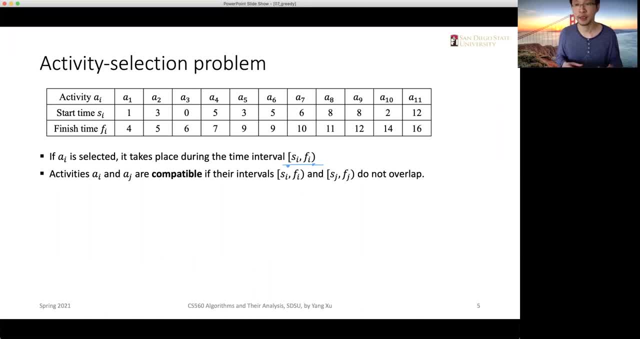 have the intervals: One is from S I to F I and the other one is from S J to F J. So the compatible- whether two activities are compatible is also well-defined, because as long as their intervals do not, 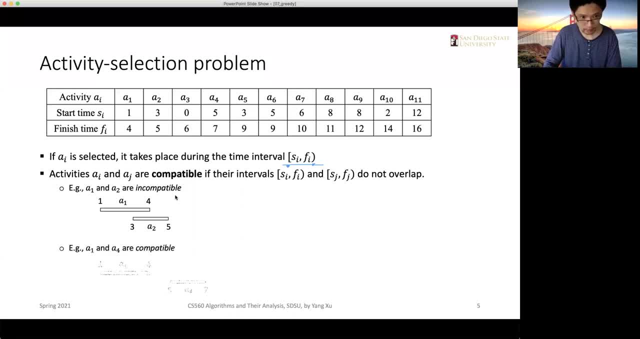 overlap in terms of the compatible. So, like the example here, if the A1 and A2 are incompatible, which means they cannot be scheduled within the same day, then it's simply because if we look at A1 and A2, the 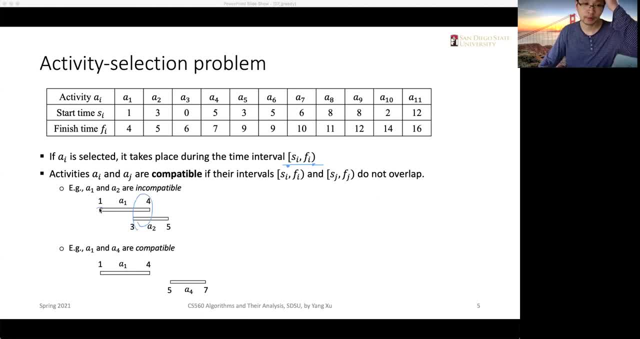 intervals: right, have an overlap, And at four, but the A2 starts at three, which is before two o'clock, right? So there's no way to schedule A2 while A1 is still going on, right? So? 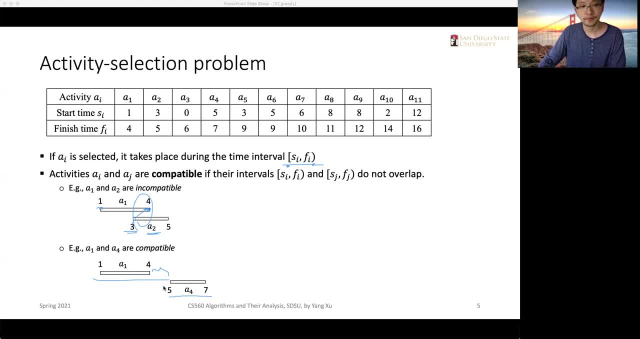 unless the A1 and A4, like these two activities are very far away, like they never overlap, okay, So these are just examples. So, generally speaking, we can compare the starting time with the starting time of one activity. 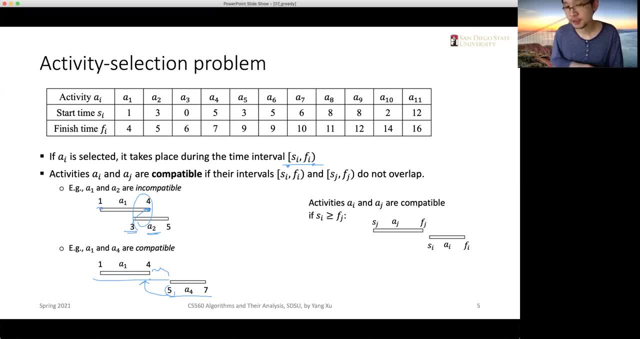 with the end time, the finish time of the other activity, Say, if the starting time is finished, then apparently this case is a compatible case. Or in other case, if the it's other way around, If J. 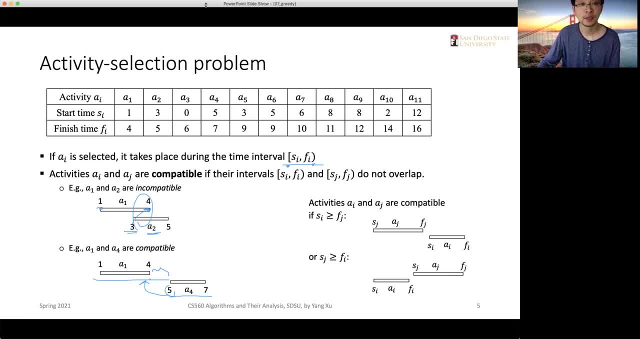 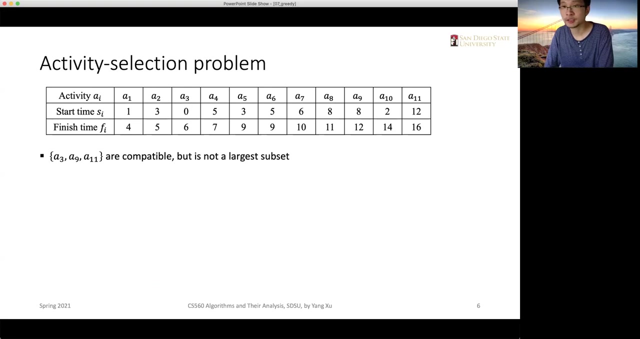 starts after I is finished, then that is also okay. okay, So this greater than or equal to relationship if we actually happens later. okay, So that is our rule of defining the greater than or equal to relationship. okay, All. 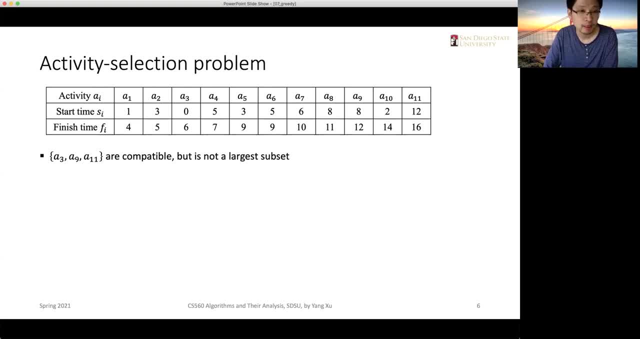 right. So in this particular example, let's say, we just picked A3,, A9, and A11, here, So they are actually compatible. okay, But unfortunately this is not the largest subset, which means we are. 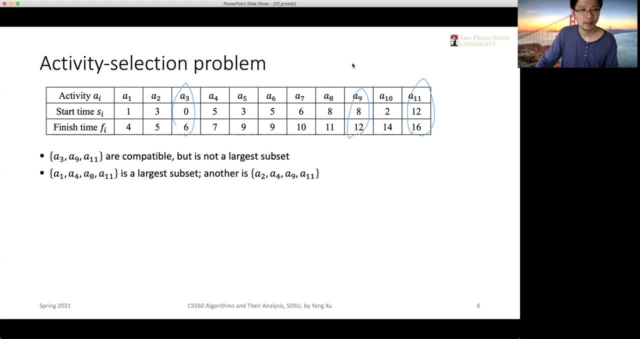 not scheduling as many activities as possible? okay, And actually, if we look at A1, right, A1 starts at 4, and A4, right Starts at 5, and at 7, and A8 starts at. 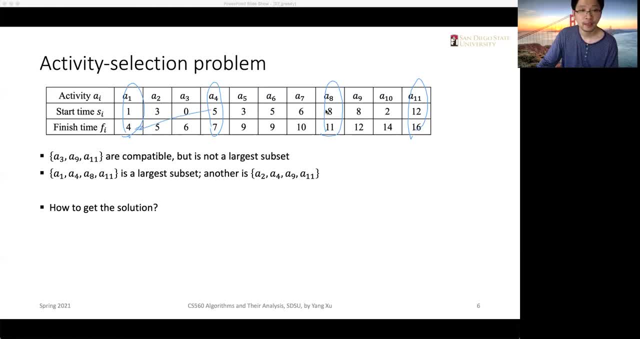 8 o'clock and A11 starts at 12 o'clock. see, So the starting time of A4 here is after the start of A7, right, So we can actually schedule four activities And in this particular example, 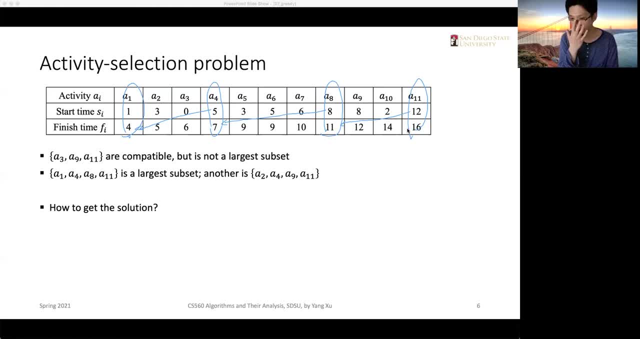 these four are the largest subsets, okay. Well, there's another option, which is A2, A4, A9, A11, okay, So it's like it's decided by the goal is like schedule as many number of activities. 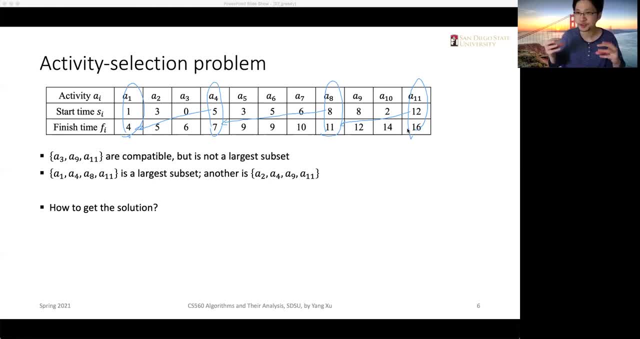 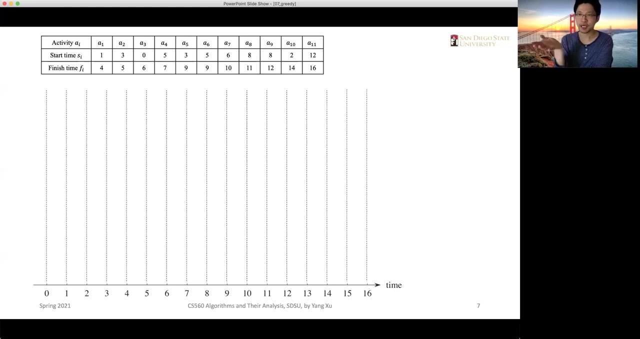 as possible, It's not as longer time as possible, okay. So it will be a different type of question if we have the same number of activities in the same time. So actually this problem can be like it's pretty like visualizable. 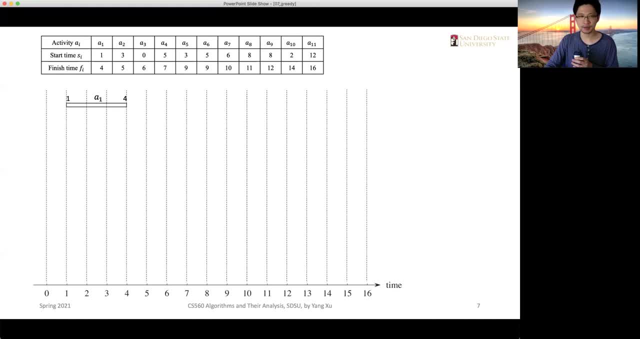 Like if we plot the resource, which is the time we have here, say we first, we just layout all the activities, we just plot all the activities on this vertical, I mean horizontal line of time right, Horizontal line of 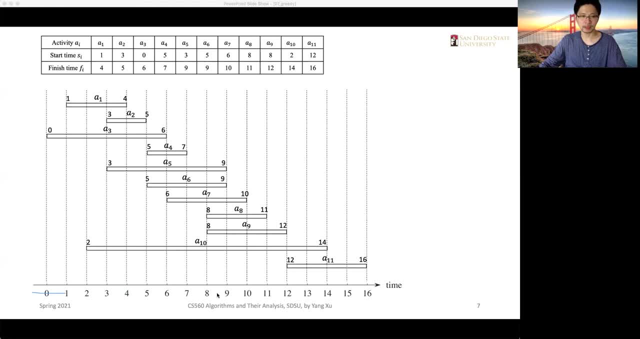 time which, at the bottom of this plot, plot each activities and let them stack onto each other. Okay, so that it's very easy to observe whether we're gonna have an overlap in terms of occupation time. right, So let's start by. 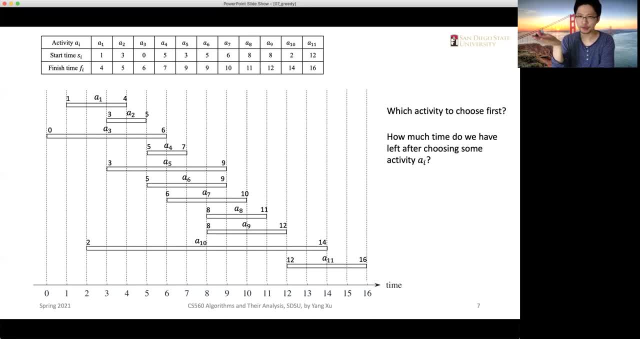 asking a question: Which activity do we choose? Okay, because choosing an activity will have an outcome right After we have scheduled, after we have chosen this activity, then we are actually removing some time out out of our pocket, out of. 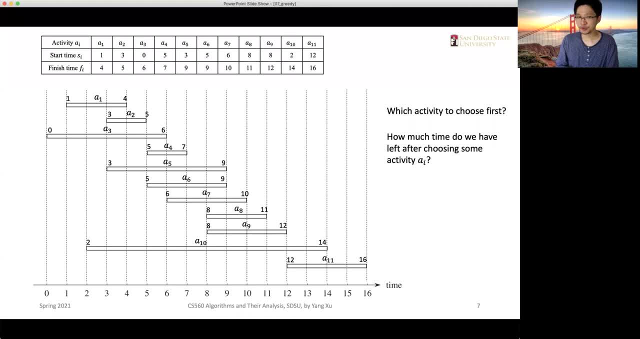 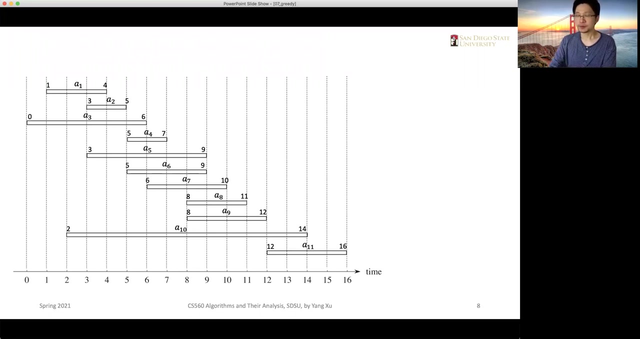 our pocket. So we need to consider this outcome of choosing an activity. Okay, so now let's consider this outcome by thinking about how much time do we have left after choosing some activity? AI, right, Because let's say, let's assume that we. 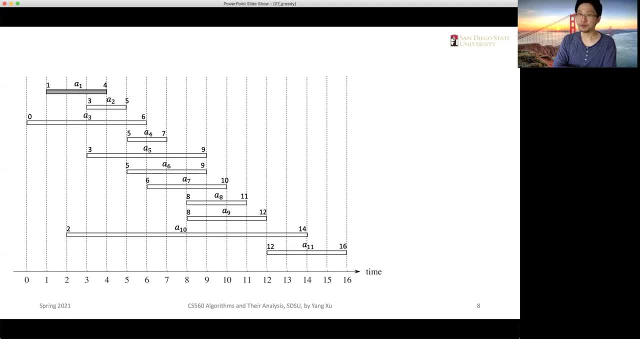 select A1, right. So now we mark it as the gray color, then A1 is scheduled. then, because A1 ends finish at four o'clock, then if we look at the time scale we only have 12 minutes right. 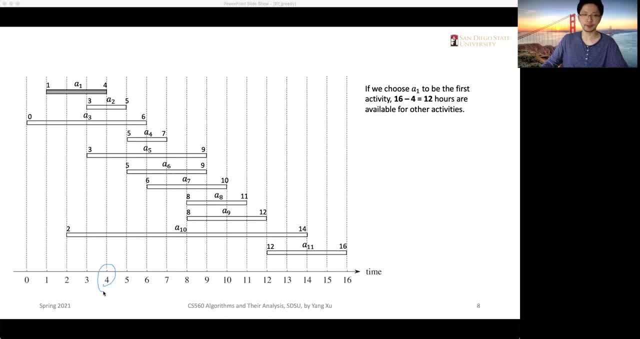 Based on the principle of compatibility, right? That is very straightforward. We only have four to six, four o'clock to six o'clock, available. Okay, so now our problem is changed. So now we are considering the remaining parts, not the original. 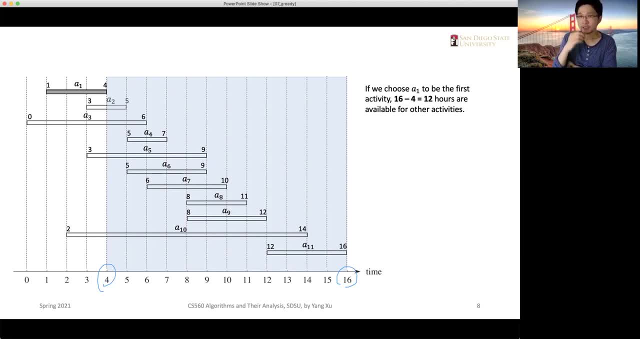 problem. we're considering the remaining parts. So what can we choose next among these available resources from four o'clock to 16 o'clock? right, And we choose so. so well, that is the outcome of choosing A1 to be the. 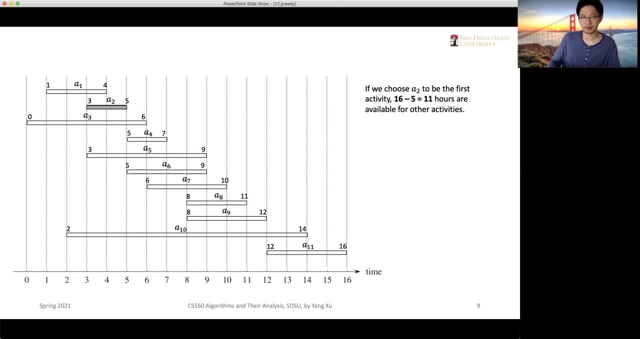 first activity right. Then from five o'clock to six o'clock, 16 o'clock, which will be 11 hours that are available to other activities, right, And it makes sense to look at all the other activities, right, Because 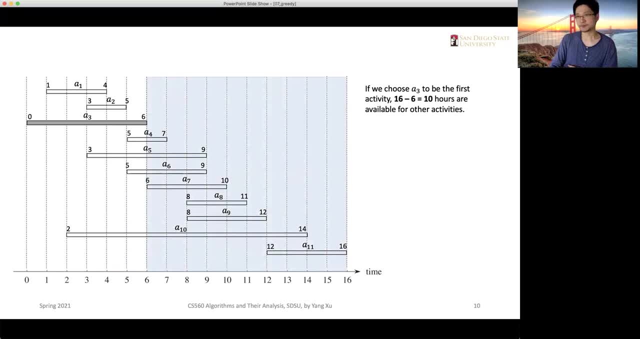 A3 ends at six, so we only have 10 hours left, right. So that clearly shows that we have different outcomes and we choose different activity as the first activity. okay, So the last activity, then it will be a. 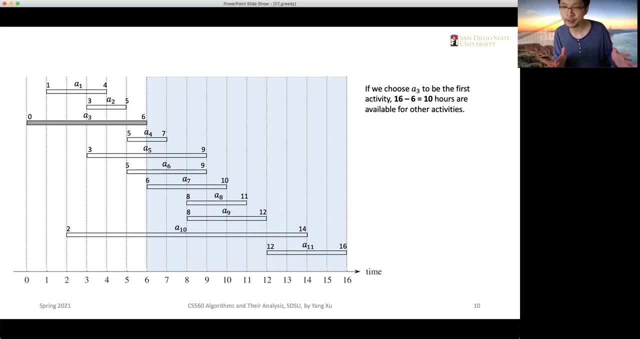 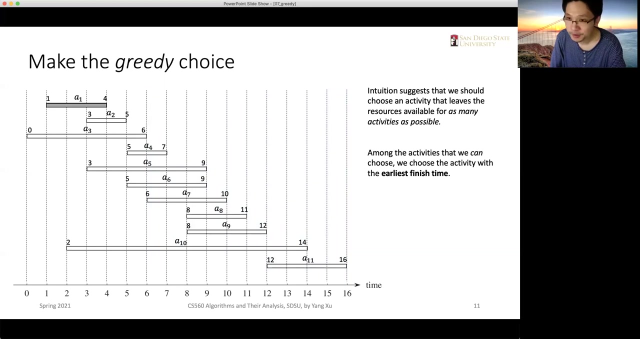 different thing we need to consider. We need to consider what's the available time before this activity starts right. So you see, it's interesting to know that we have different options, So we choose different activity first. okay, All right. 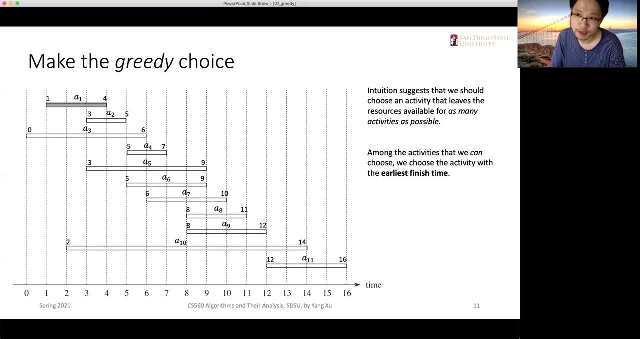 So now we are almost there to come up with a solution, with a strategy at least. okay. So actually our intuition is that if we choose A1, and then there's 12 hours left, or we choose A2,, 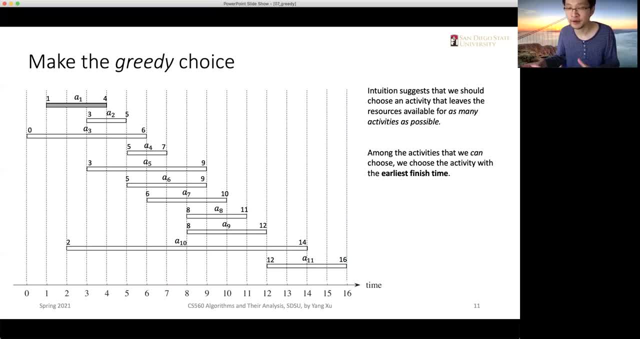 but there's 11 hours left, then our intuition is that, okay, I will prefer to choose A1 because we have more resources left. okay, So why not? we just stick with this intuition And whenever we can choose among activities. 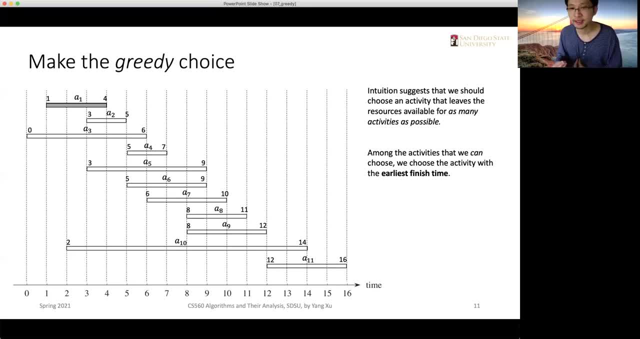 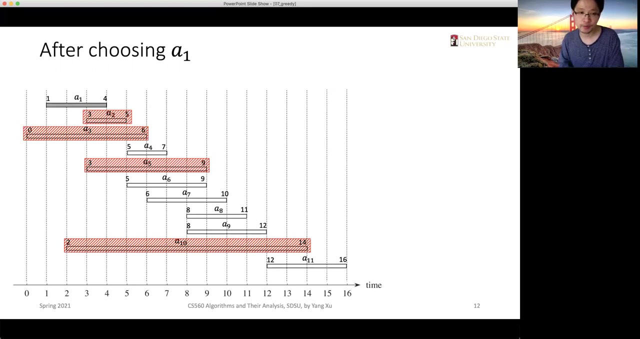 we can use this intuition to guide us. We can choose A1 to complete the solution. okay, So let's work on this example to complete the solution. okay, So let's choose A1.. Then what happened? is that A1? 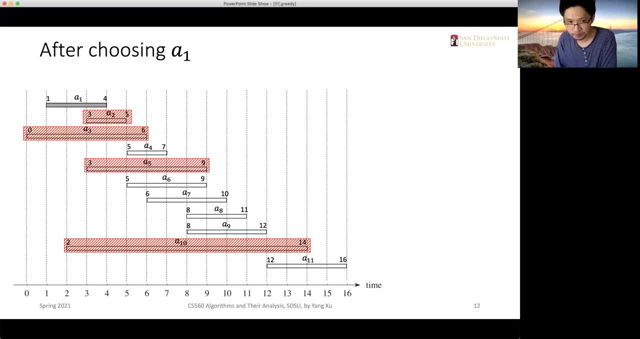 is one of the remaining activities. right, There are some activities that cannot be chosen because they are not comparable with A1, okay, If you look at A2, it starts at 3 o'clock, but 3 o'clock is the time. 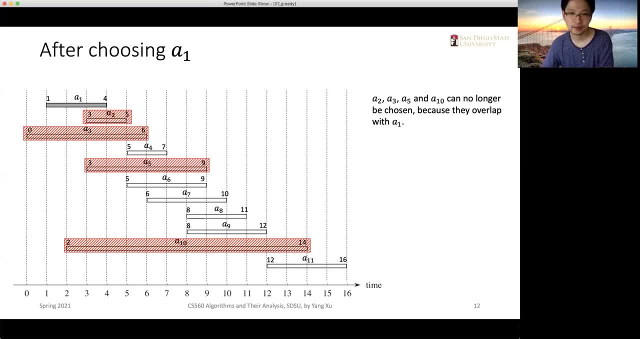 scale. So we can only choose among A4,, 6,, 7,, 8,, 9, and 11 among the remaining activities. okay, So when we choose among those remaining activities, we have to save as much time. 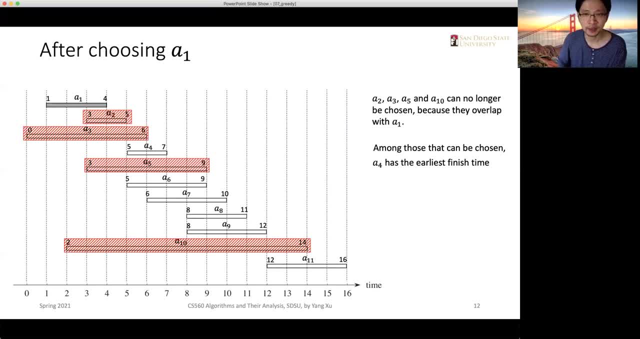 as possible. So among the remaining six activities that are compatible with A1,, actually A4 has the earliest finish time, so we can choose A4, right. So that means we can remove A6 and A7, because A6 and 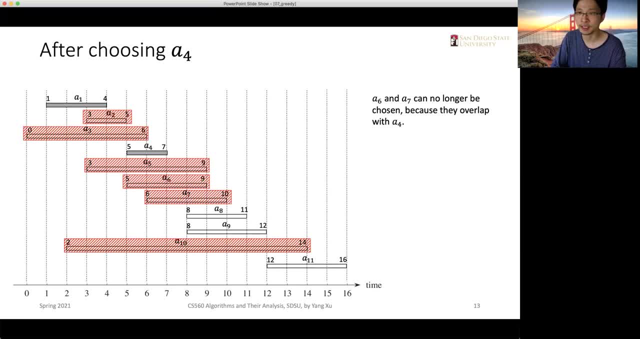 A7,. they have an overlap with A4, okay, Since A4 is chosen, then obviously we cannot choose A6 or A7 anymore. All right, so there are A9, A8, A9, and A8 in this case. 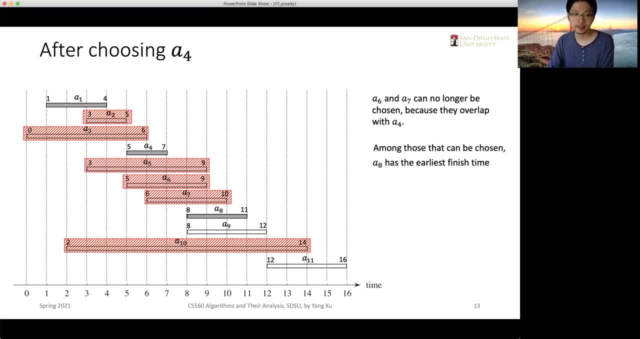 All right, so we choose A8, and now A8 overlaps with A9,, so A9 is also gone. so the remaining choice- the only one remaining actually- is A11, and so we choose A1,, A4,, A8,. 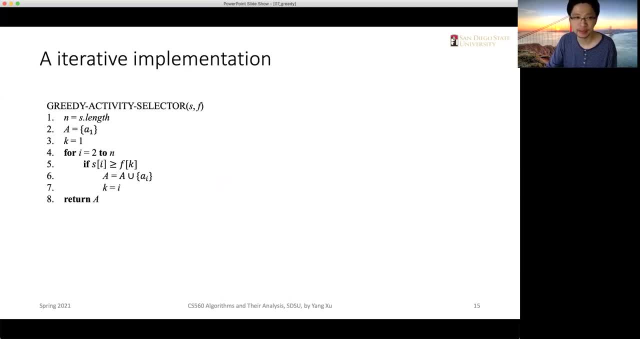 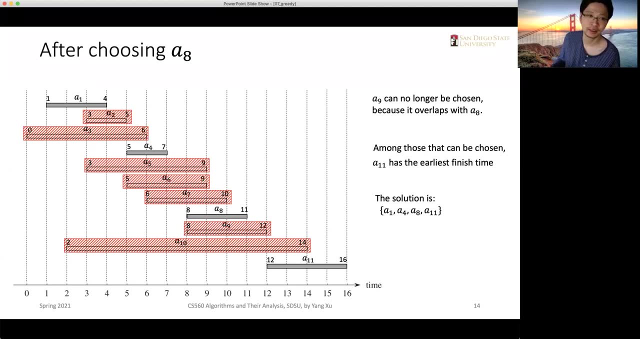 and A11, okay, So quite straightforward right. As long as we take this strategy, it's quite easy to get at least one solution right. So, although this strategy doesn't mean, that doesn't guarantee that we obtain all the possible, 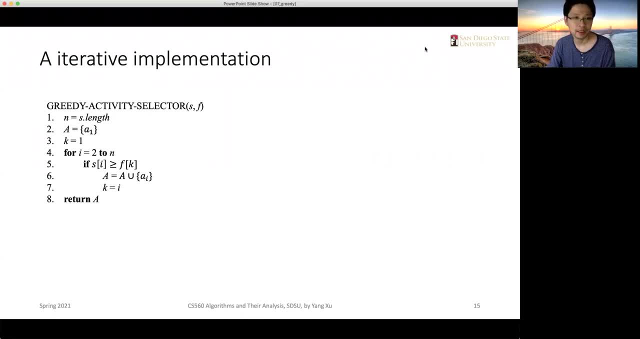 solutions, but it is one solution, right? All right, let's look at how we can actually implement this solution. okay, So let's look at this recursive implementation as well. Anyway, let's look at this greedy activity selector, this procedure. 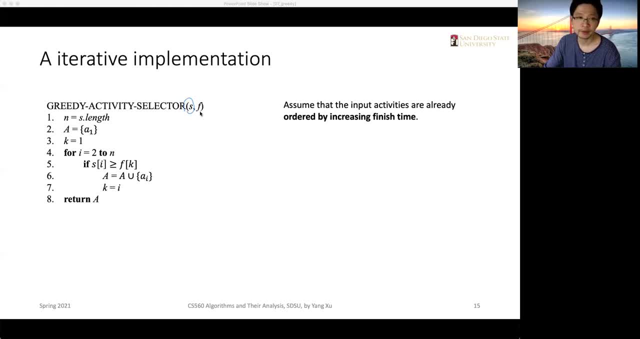 okay. So this procedure: it takes inputs- the starting time and the finish time- into the end time. Okay, so this implicitly says that we need to sort all the activities first, which comes with some additional costs- additional running time costs. So 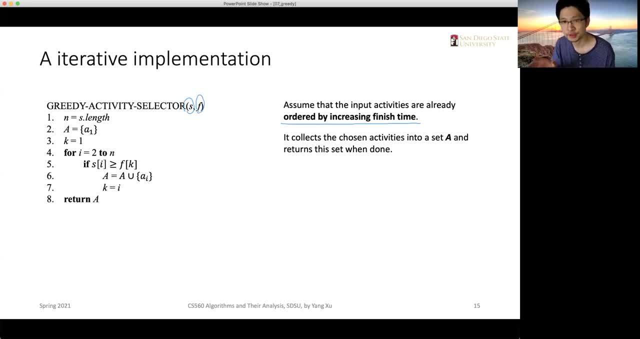 that's important to keep in mind. with All right, so let's look at the remaining code, And this second line of code actually simply initialized the sets with A1, okay, Because A1 must be chosen, because it is the first line of. 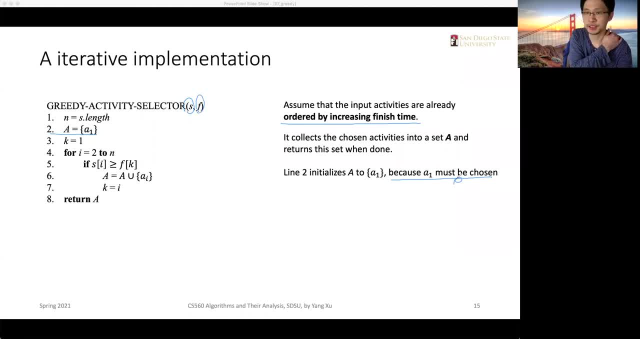 the first activity: okay, And the K. actually. it's an index that indexes the most recent addition to the set. A, okay, And the case elements in F. F of K is the maximum finishing time of any activity in A, because it's. 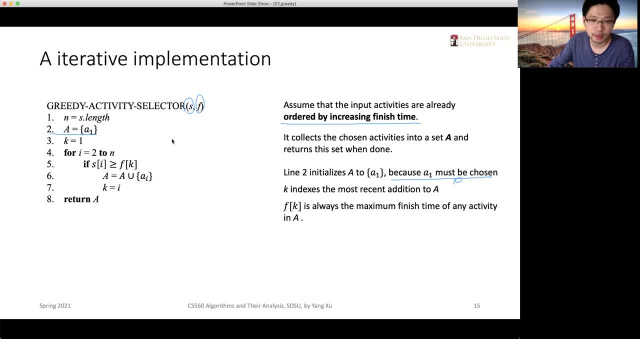 the most recently added elements to the set A. okay, So if we look at line four to seven, it's a set of two parts. after A1 is selected, right After A1 is selected, we need to iterate from two to N. 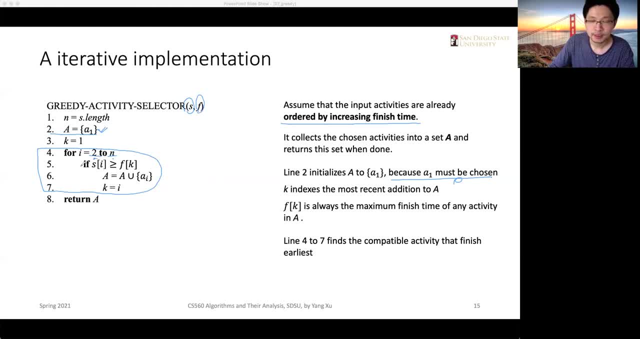 because we have N in total. okay, So within this for loop there's an if condition. okay, It checks the set A, that is, within this set A. okay, Because at the beginning K is one. So at the beginning, 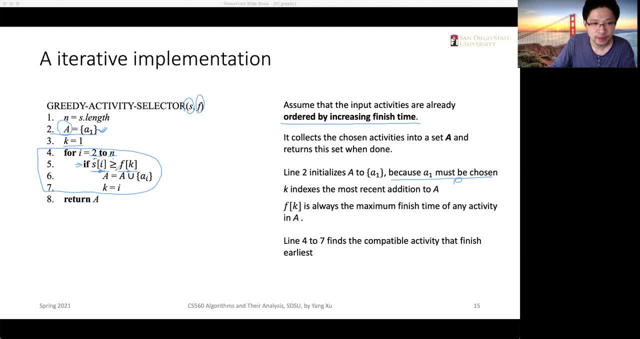 so this FK is just F1, okay, Which is the finishing time of the first activity. okay, So if this condition is A, which means the activity I is a compatible one, right, Because it is compatible, we need to select it. 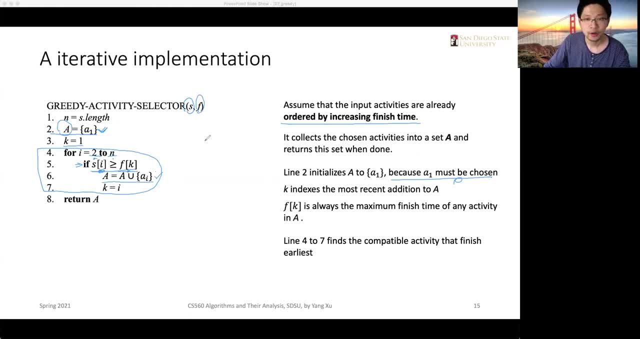 okay, And that's also because all the activities are ordered by the increasing finishing time. okay, So the first one, the second one, the third one, the fourth one, the fifth one, the sixth one, the seventh one, the eighth. 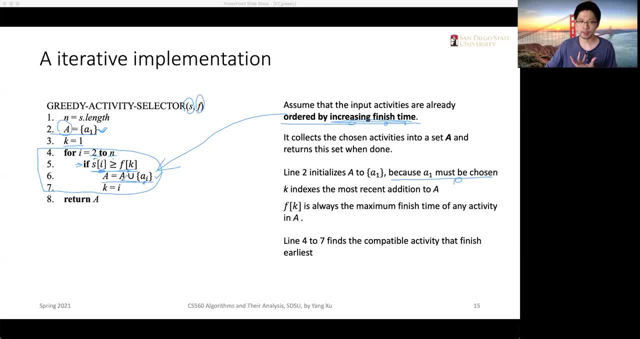 one, the seventh one and the eighth one and the ninth one, the seventh one and the eighth one, so the next one. we are going to compare the new I with the FK, so this FK would be the first one. 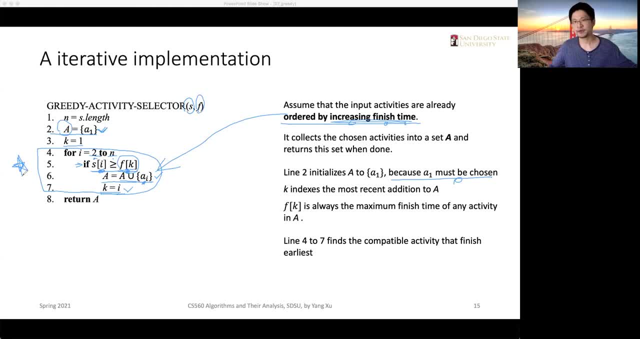 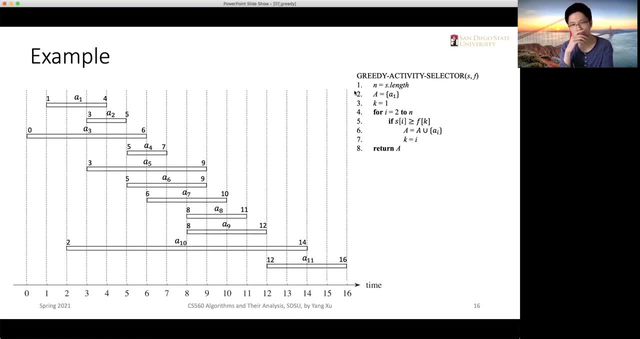 and the second one is the third one and the fourth one is the seventh one and the eighth one, the seventh one, the eighth one and the ninth one, and and the last one and the last one, the sixth. 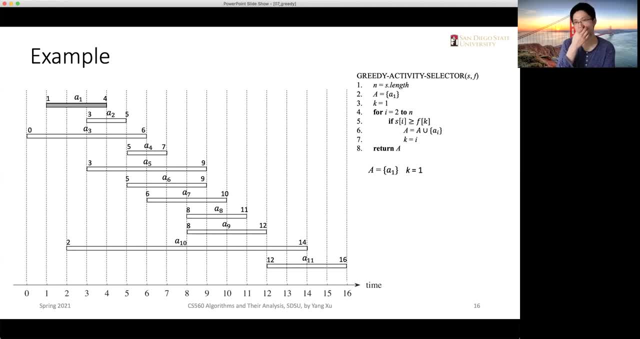 one, the sixth one and the ninth one, so the important one. the second one is A2 to N right, So I will be first two, okay, But now, since A2, if we look at S2, so this is S2,. 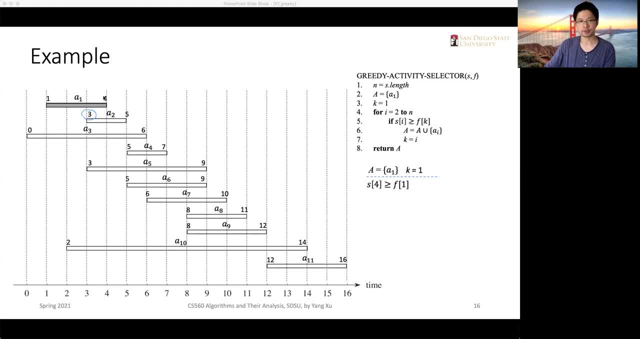 right, The S2 is three, which is not greater than the F1. So let me write F1 here, So the F1 is four, right? So the S3 here is smaller than F1. So A2 will be incompatible, right? So next we will have: oh see, it shouldn't be S2, but it should be. 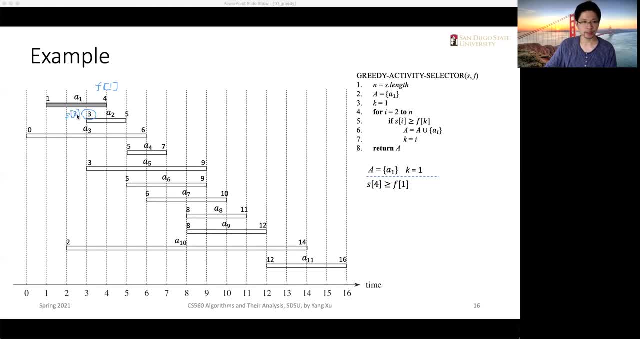 S2, right, Not S3. There should be S2. And this zero would be S3, right. It's also smaller than F1. So until we have met A4, which is S4. here, S4 equals five, which is greater than. 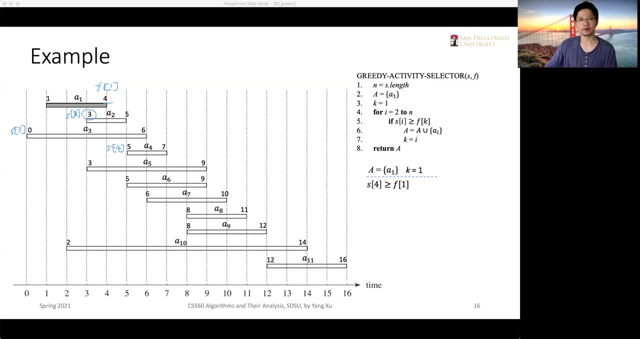 the F1. F1, four here. So A4 would be the one that we incorporate into the set A, And then we need to update the K to four. So from the next iteration on we need to compare the SIs with this F4,. 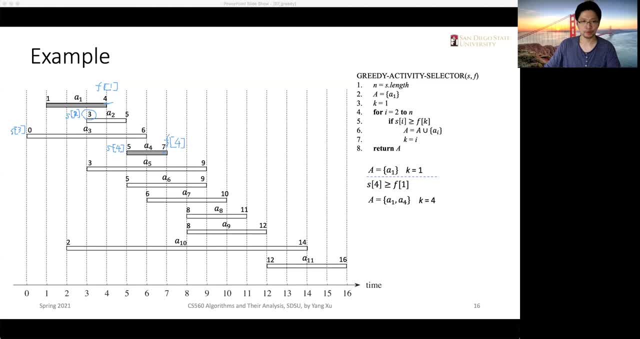 okay, Because we need to see which activities are compatible with this new finish line. So that's the finishing time boundary, finishing time condition: okay. So of course, A5 is not compatible. Six is not compatible because we're comparing these with the F4, right, With the F4.. 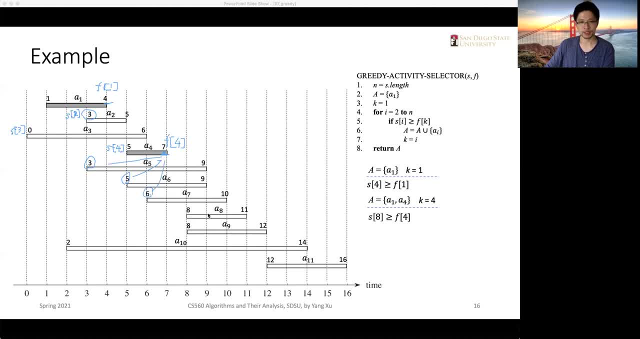 And this is not compatible until we see the S8 here. S8, right, S8 is eight o'clock, which is greater than, which is greater than F4.. a bingo: here we need to select a8 into the activity, into the sets. okay, and then updates. 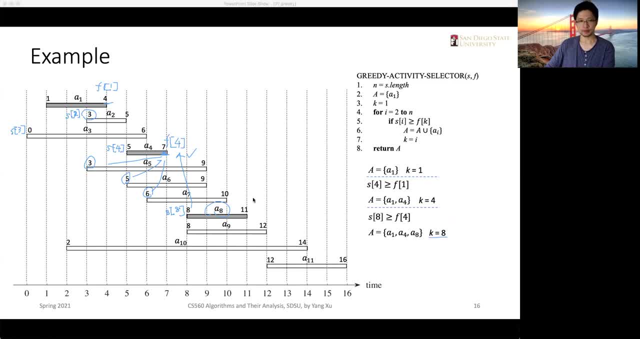 the k to be eight. so now we will set this f8 to be the one that we are comparing with. all right, so until we have, lastly, uh incorporated the activity a11, then we have, uh, basically everything solved, right? that's pretty much very close to the strategy that we described at the beginning, right? 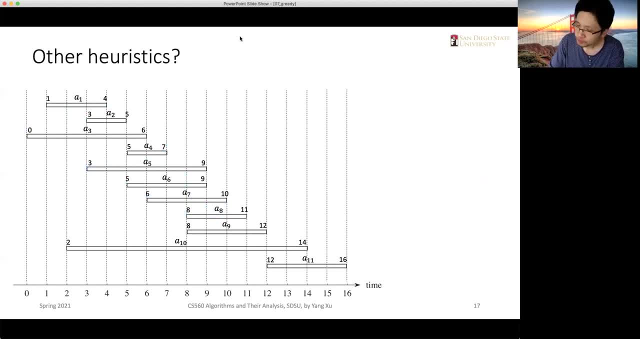 all right, that's an uh um one uh, uh, iterative, uh, implementation of the algorithm actually. so can we have other heuristics? i mean, uh, the currents current heuristics that we use is the one that has the earliest finishing time, right? so what about, instead of choosing activity with the earliest finish time, what about we? uh? 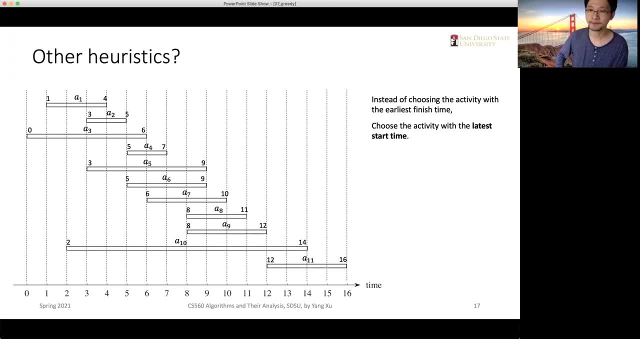 choose the one with the latest start time, right. that is also, uh, a different way of thinking, right, it's a kind of backward right. we will start from the one with the latest start time, right. say, it's just a backward thinking we, we select a11 right and 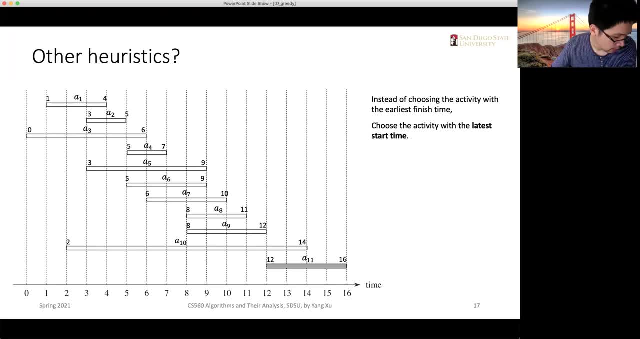 uh. after a11 is uh selected, we will similar to the, to the, to the forward thinking right. we will have a um, a changed uh space of selection right, because 11 is chosen, then we now we can only consider those that uh finishes before the uh a11 starts, which is 12. 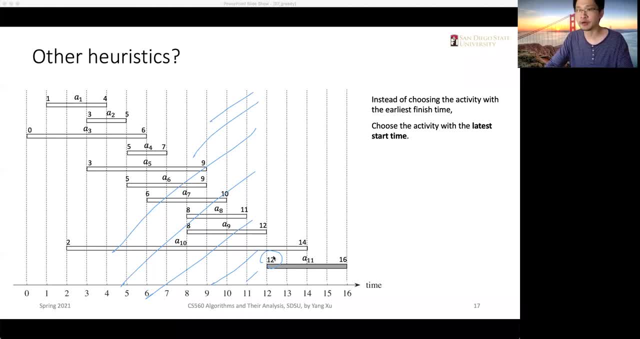 then we we need to only consider the space before 12 o'clock- before 12 o'clock, right. we need to consider those activities that finish before 12 o'clock, right. it's just the other way around of of solution. then 12 i use for 12 o'clock as a threshold. we need to choose the one that 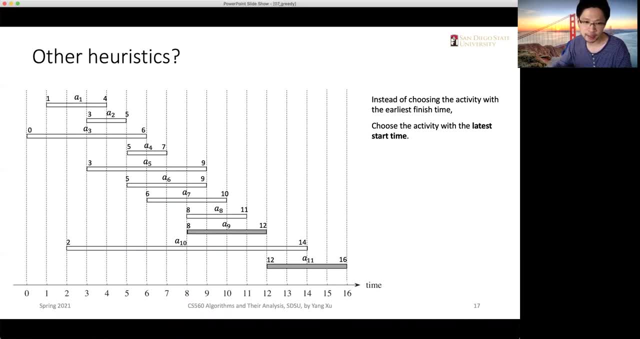 has the latest start time, which is a9. right, because a9 has eight o'clock at start time, and that is the first one we came across. so a9 would be selected and the a9 is selected, and then we need to choose the one that has the latest start time, which is a9, and then 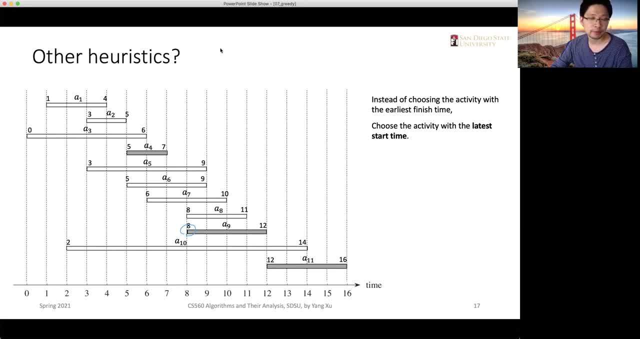 it. we will have the remaining parts among the remaining uh activity. we can choose a4, right, and a4 is chosen and a2 is also chosen, then we will have a2, a4, a9, 11 as a way to uh, as a, as just one selection, as just one solution to the problem. so, uh, so far it's so good, right it? 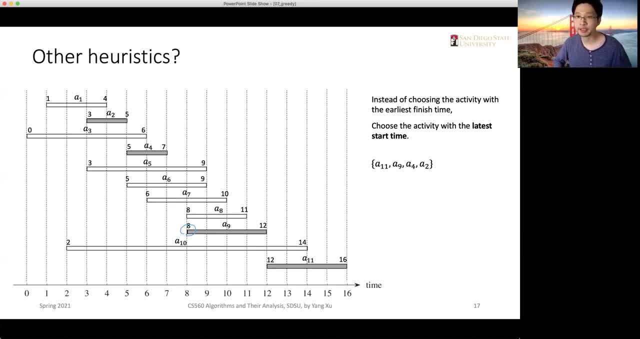 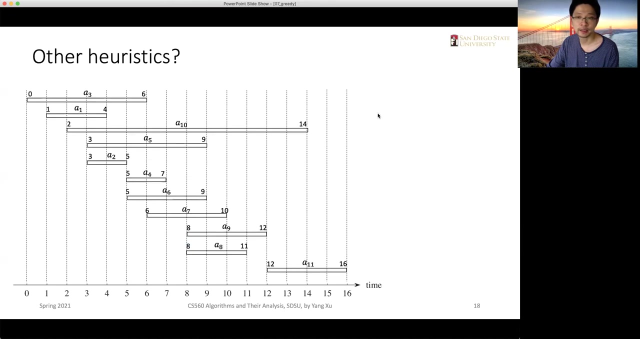 looks uh, close, it looks correct, right, because it's also scheduled uh for activities for us actually, but this, um, this way of thinking, in this condition, in this uh particular example, it's not, uh, totally correct. uh, because we, we didn't, we didn't look at the conditions yet. okay, the the condition. 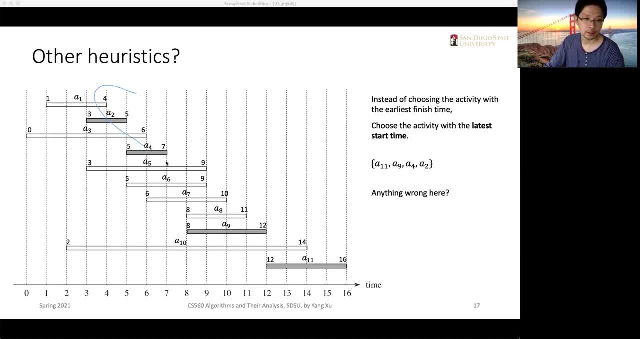 is that all the activities are sorted by this finishing time. okay, so the activities, they are ordered, like by the finishing time, from four, five, six, seven, nine, ten. right, so that is an order of the activities. if we use the latest start time as our heuristic, then it actually doesn't work with this. 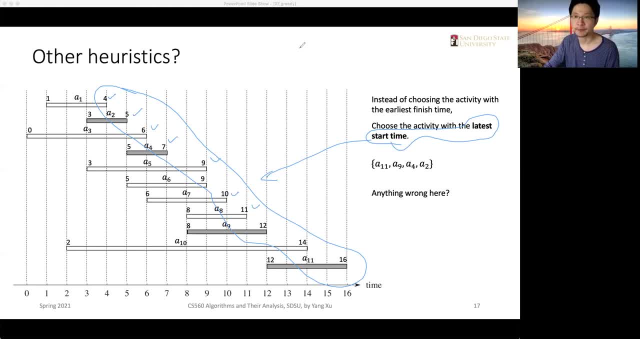 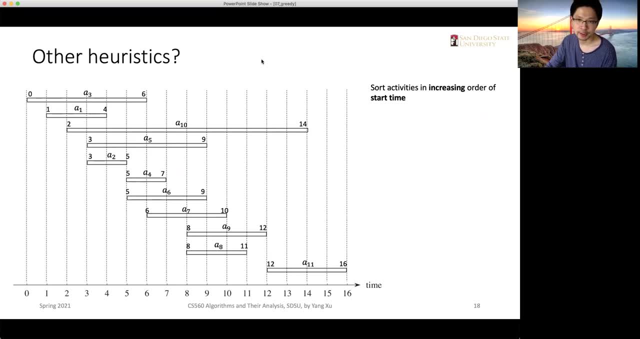 uh sorted time with uh finishing time. okay, so the the sorted activity with finishing time. we actually need to sort them. uh, regarding the starting time: okay, so, for example, let's uh look at this problem: if we sort the activities in increasing order of the start time, right then the activities would be in a different order now. 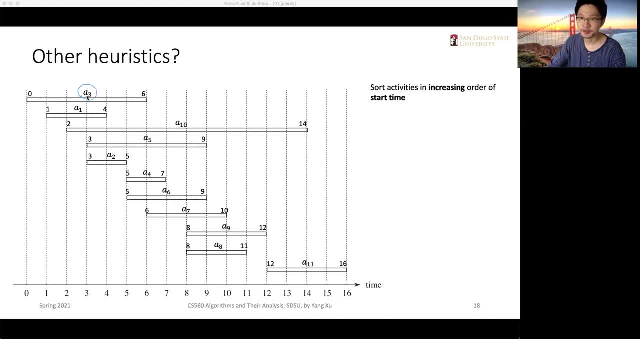 a3 would be the one that starts first, not a1. okay, because a3 has a zero clock starting time. then it will be a1 and then a10. right, because a10 starts really early. okay, so assume that we sort all the activities in such an order of, uh, increasing start time. 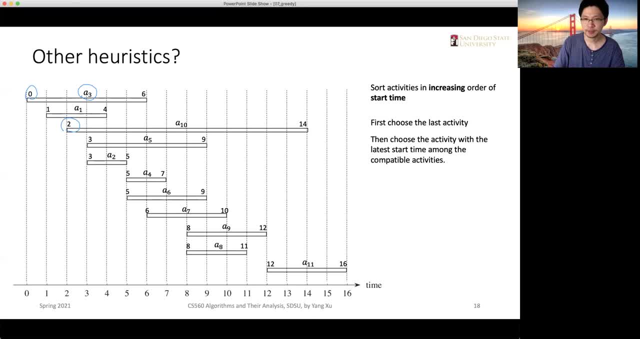 then we first choose the last activity right, which is a11. right, let me clean up. so we need to choose a11 first, Okay, and then we call in the 3.ここ等点 加後时间. we need to choose the activity with the latest start time among the compatible activities. 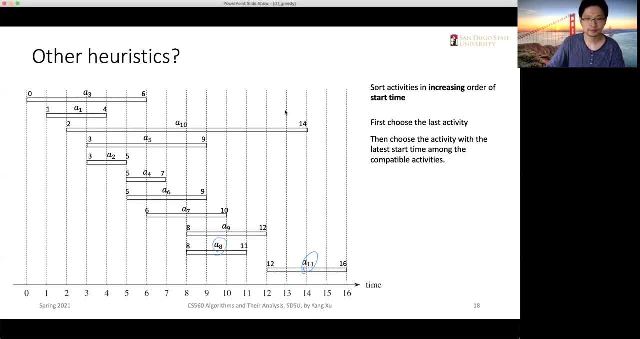 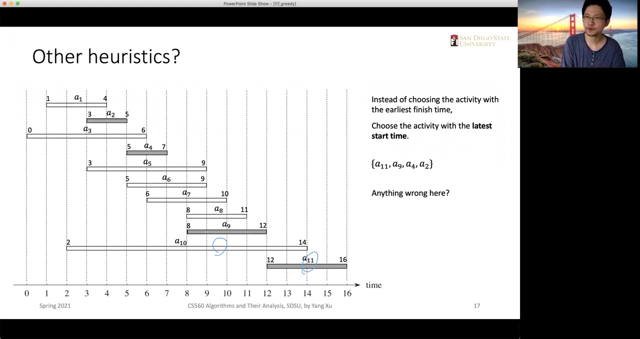 which would be A8 and A4 and A2.. That is, A2, A4, A8, A11.. Okay, so this heuristic. this second example. it actually doesn't differ too much from this previous slide. We also have four actives selected. 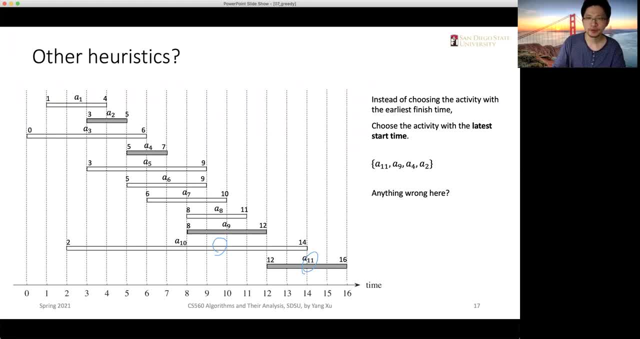 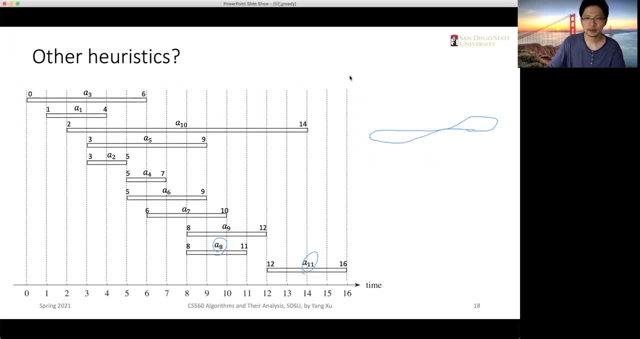 So what if we choose the? what if we use the heuristic that we select the latest start time with in the second example here, after we have sorted all the activities in the increasing order? Okay, Oh, okay, that's exactly what we did. Okay, all right, I made a mistake. 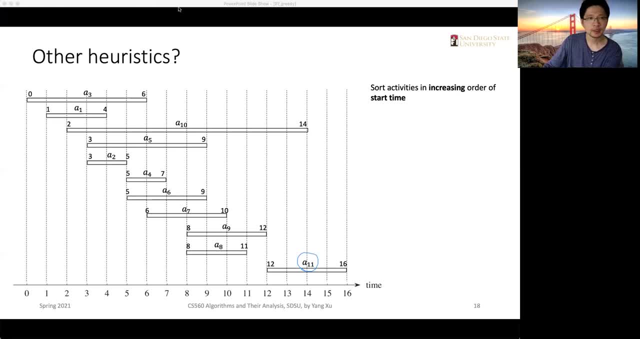 So we actually chose A11 and A4, A8, A4 and A2.. Yeah, that's correct. So what I mean is that this way you of choosing the latest start time is only correct if we have sorted all the activities. 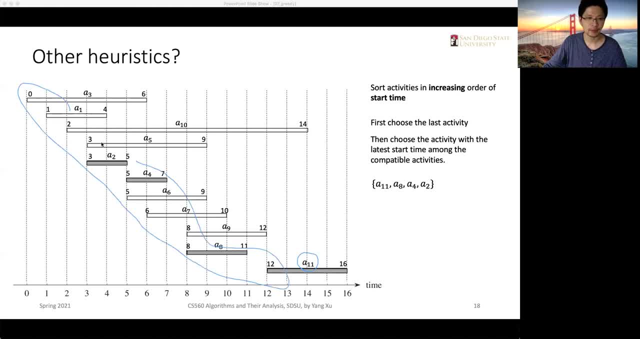 with the increasing order of starting time. Okay, it doesn't necessarily work if we start, if we choose the one that has, if we sort all the activities that with the increasing finishing time, Okay. So yeah, I probably I should write a counter example that's showing that. 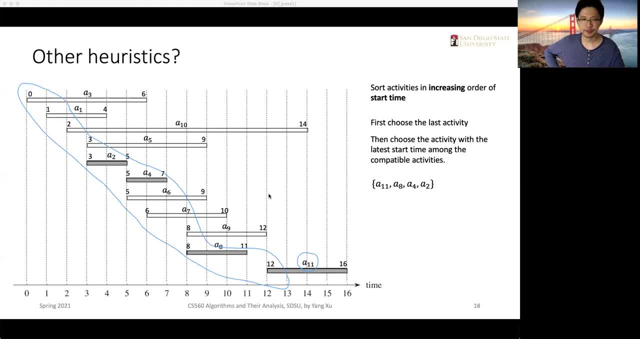 if we sort the activities by increasing finishing time, then this heuristic will not work. Okay, but I didn't have this slide here. Okay, so I'll look into this, so probably I can provide a counter example next time. Okay, Anyway, let's. 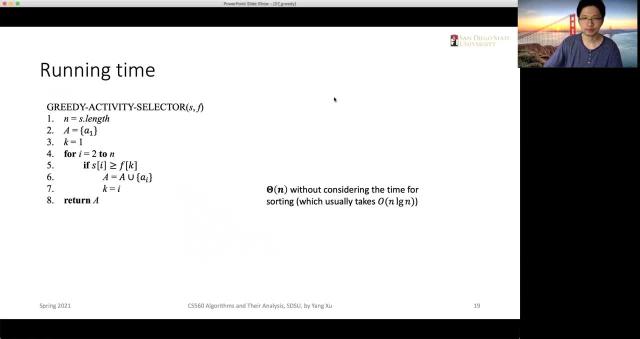 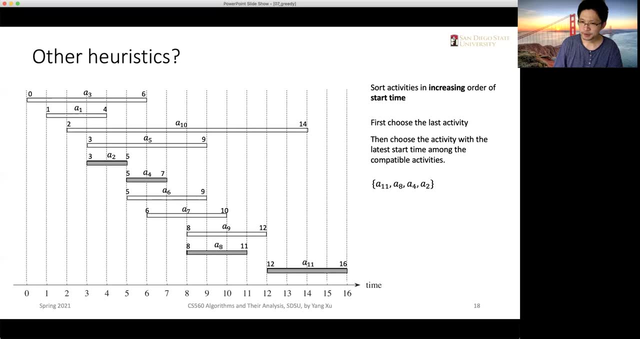 go to the next slide for further analyzing the algorithms. There are different ways. just by reference, it doesn't seem like these different implementation would affect the right time. Yeah, So spoke of running time, the. this algorithm is quite efficient actually, because it's just a iterative search over the. 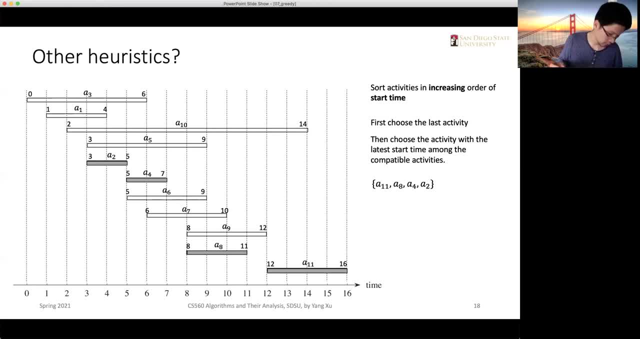 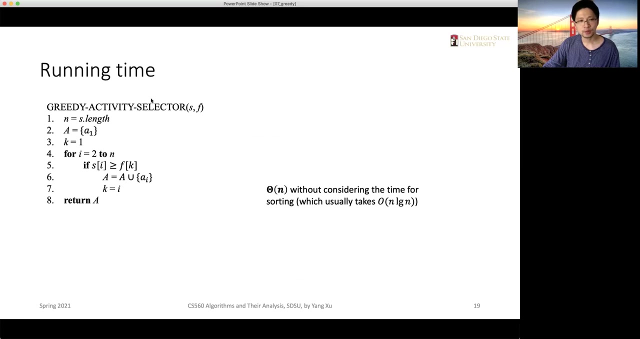 over all, the kind of a linear search over all the possible activities, Right, But the correctness is not needs to be examined carefully in terms of- in terms of how much- how the activities are sorted in order. Okay, So it's actually quite straightforward, right, because we use a one for loop to iterate. So 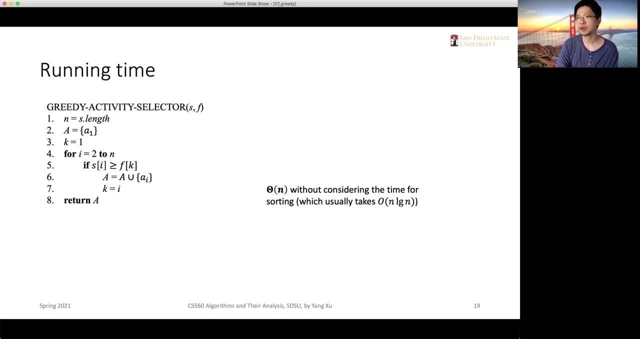 over basically almost all activities from two to n right and it's more or less it's just like big theta of n right. but actually we didn't consider the fact that we sort all the activities just before we run the the query search, query activity selector. okay, so strictly speaking, we 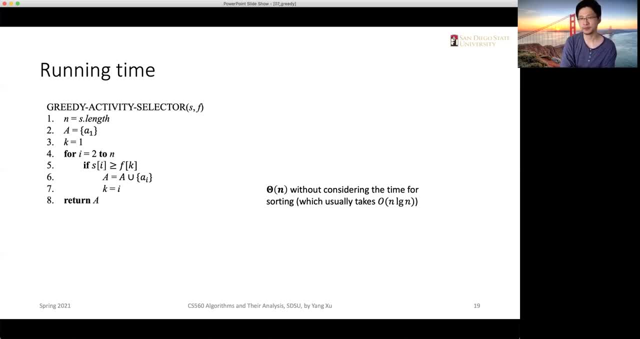 we need to say that it's at least n times logarithm of n. okay, yeah, but somehow, if we are able to solve the problems, like with some more efficient sorting algorithms, like the linear time sorting algorithms, because so far the the examples we have all have starting time as integer numbers and for integer numbers we 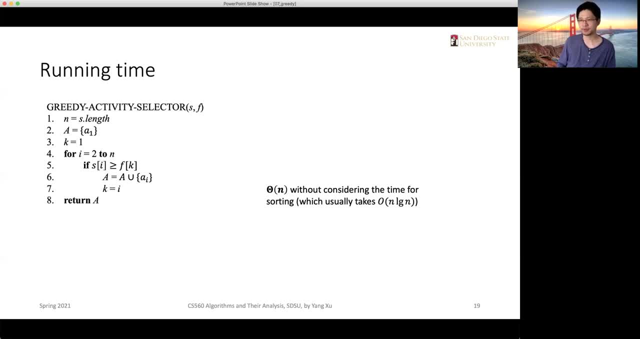 it's, it's actually, uh, we are able to apply some efficient algorithms to sort the all the numbers. all right, okay, so that's the implementation for, uh, well, the, the iterative implementation for the activity selection problem. so, uh, if we try to connect this problem with dynamic programming, 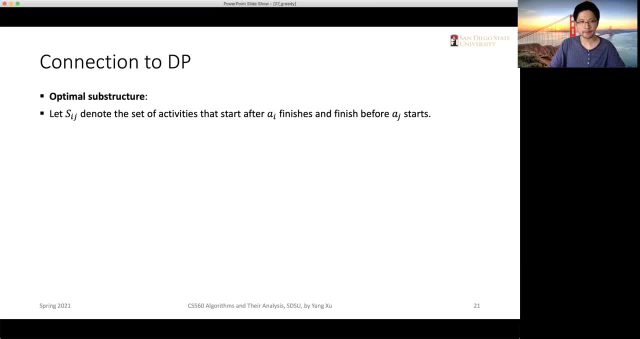 it's actually doable. so let's look at the optimal substructure here. so it's a little abstract. now we use our mathematical notations. okay, we use the capital s, with subscripts from i to j to indicate the set of activities that starts after ai finished and finished. 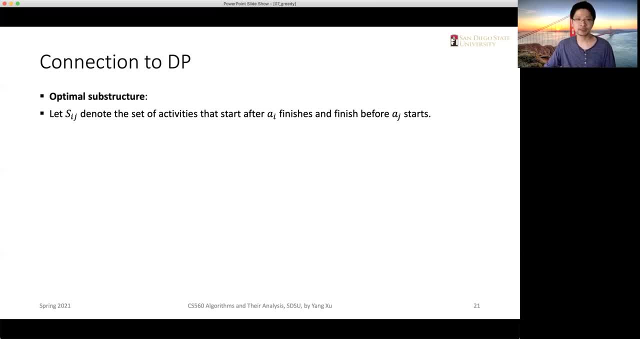 before aj starts. well, it's actually this: sij is defining some range, right, it's defining an interval or a range that starts after ai finish and the before h j starts. okay, so it's a range, and we wish to find a maximum subsets- uh of mutually compatible activities within this range. 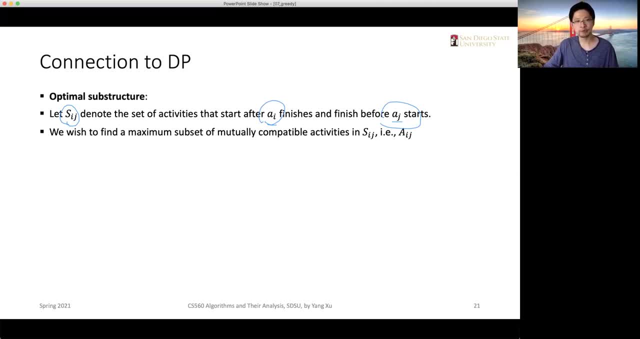 okay, so this capital s is a range, and we want to. we want to find a maximum subsets of activities that we indicate as aij. okay, so this aij is a set of activities that is within the range of sij, but we want to maximize the size of this aij. 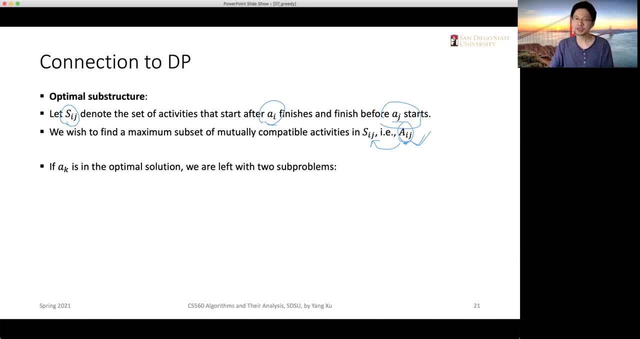 okay, and let's consider this problem. so let's assume that ak is within this solution, is within the optimal solution. okay, so actually we are left with two sub problems. you know, we like, just like the way we split, we, we divide the problem for the um, the matrix chain, multiplication, right. so we need to 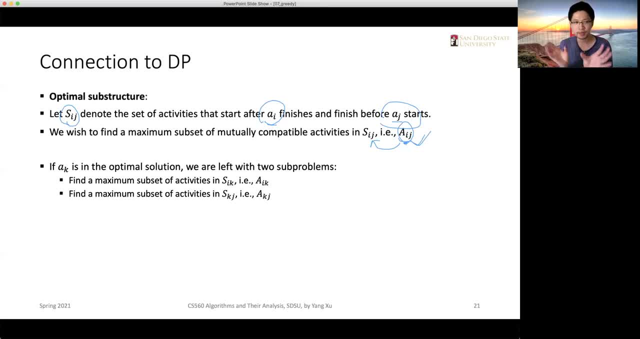 basically consider two ranges: one is to the left of k and the other is to the right of k. okay, assume that ak is already in the solution. then we need to find we need to first look at the left range, which is: uh, start after ai finish, but finish before ak starts. okay, we need to do this. 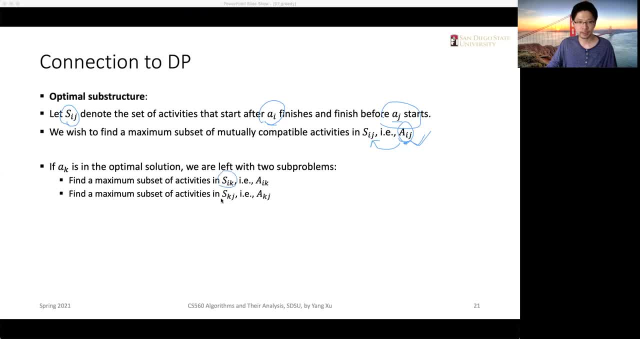 sij is the left range and this k skj is the right range, which is uh to start after a k finish. okay, so let's indicate the solutions to these two ranges as aik and akj. right, we given ak. we have split the original problem into two segments, into two sub problems. all right, so it's just uh. 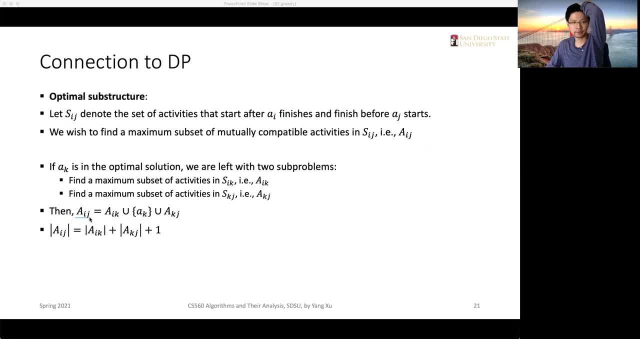 such a relationship we can extract easily, right. so the original problem is the composition of the left sub problem plus the activity in the middle. okay, so ak is in the middle and then, plus the sub problem, the right sub problem from k to j. okay, okay. so if we, because a's all the capital, a's they are sets, so we, when we describe the size of 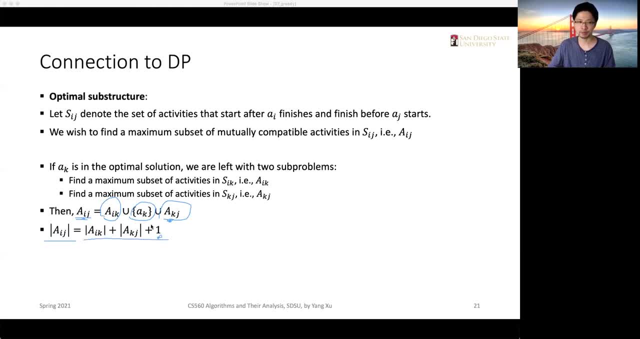 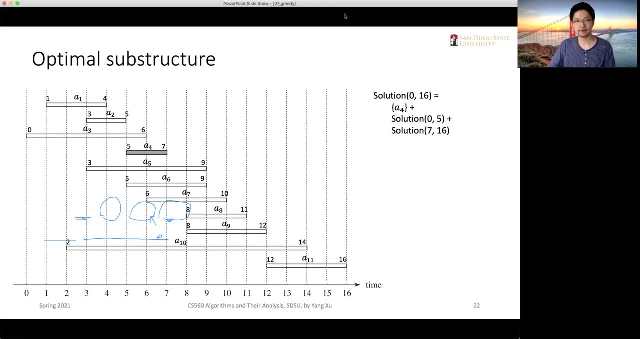 the sets. they are in such a relationship we need to plus one. this one is for this single element set, ak. okay, so it's actually a very obvious subtimal, uh, sub optimal substructure. okay, let's say, uh, now we are defining some- uh, magical functions again. right, that's the typical way of how to come up with a solution for dynamic programming. 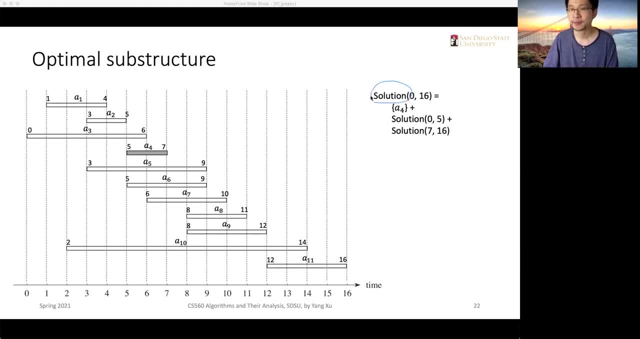 algorithms. we use this solution to indicate the, a magical function to find the solution between the range of 0 and 16, right you, we use the. this to indicate the original solution. so when we assume that we select a4, so this is a random selection, okay, on this slide it's just a random selection. so if we select a4, 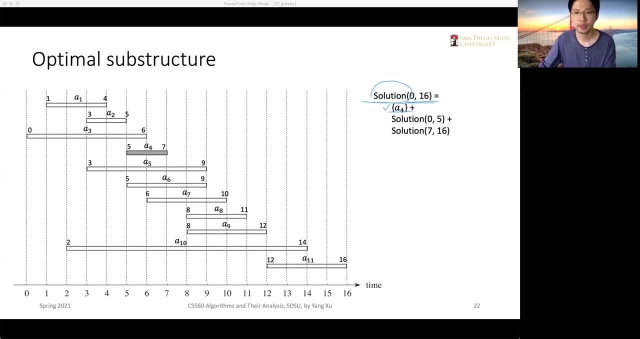 into the sub, into the final optimal solution. then we need to solve the right, the left sub problem, which is from um zero to five, which is the to the left of a4, and the right sub problem which is from uh seven to 16 right, which is to the right of the range. okay, so this is a typical uh sub, optimal sub sub. 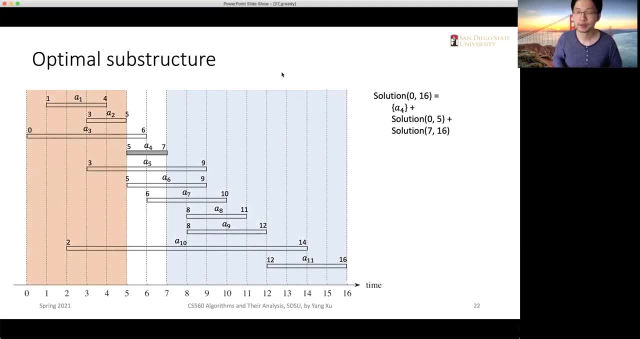 optimal substructure. right, so we are considering two ranges. after a4 is selected, there's two regions we need to consider. okay, because there's there's space to make further selections on both sides. okay, right, in this case, we are lucky to get another uh optimal solution, which is a. 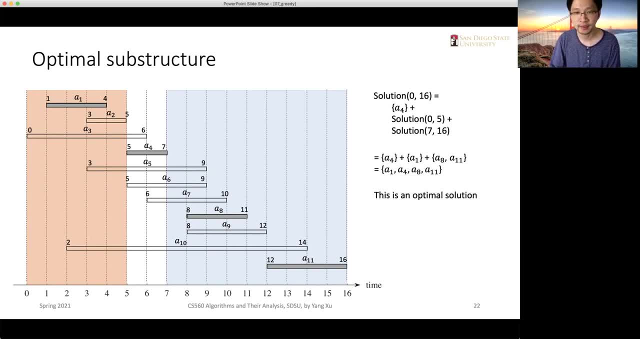 one, a four, a eight and an eleven right. so this is an optimal solution. okay, but what if we select a5 as the central activity? then to the left we have to the right we have uh from nine to sixteen and to the left we have uh from zero to three. that's also two regions to select. okay, but this time we 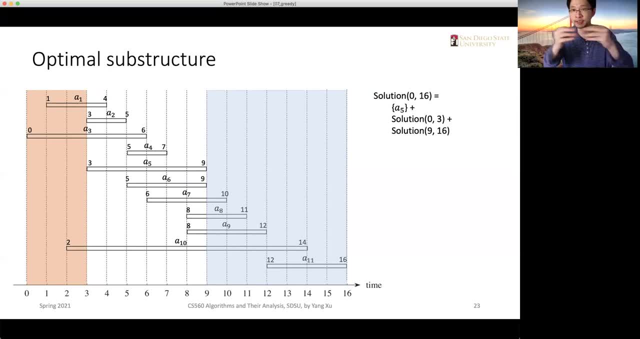 are not lucky, because a5 is too wide and it cancels the range of the sub problem, which is a five to out a lot of space. So if we choose A5 first, then there's actually only one compatible activity left, which is A11, right? So in this case the solution becomes A5 and A11, which is obviously not an. 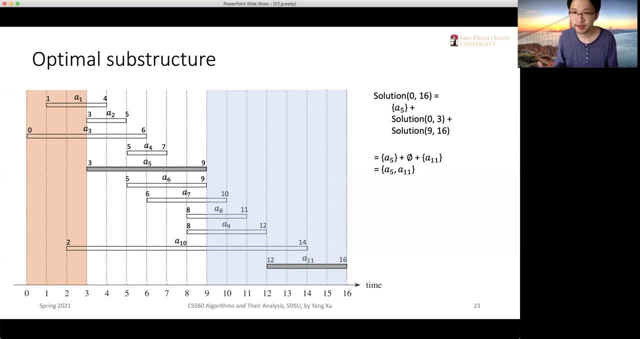 optimal solution. okay, So how do we find, how do we list, how do we get all the possible, all the optimal solutions? We need to basically iterate over all possible sub-problems. right, Because choosing A4 is different from choosing A5 first. So we need to look at how our initial selection. 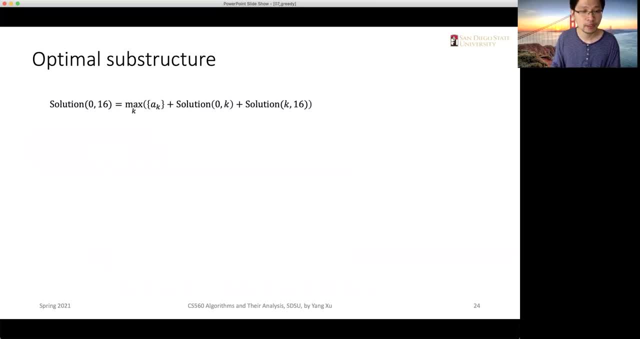 gonna affect the remaining parts. right, So we simply need to iterate over all possible AKs. So AK would be the one we first select. right, We need to iterate over all possible case. right, The solution would be AK, the union between AK and the solution to the left and the solution. 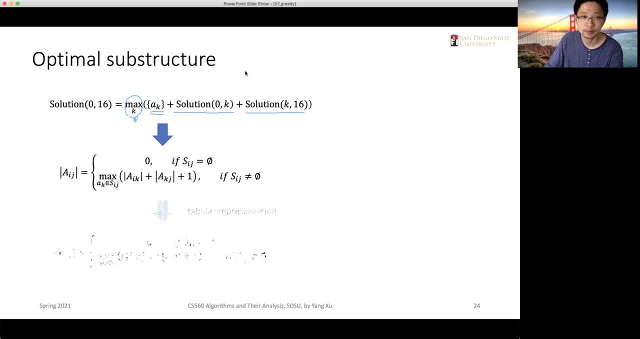 to the right. So this is a very typical dynamic programming thinking right And the recurrence would be like this: right, We need to use the size of the left sub-problem to the plus the solution to the right sub-problem, plus one right. That would be the solution to the original problem. 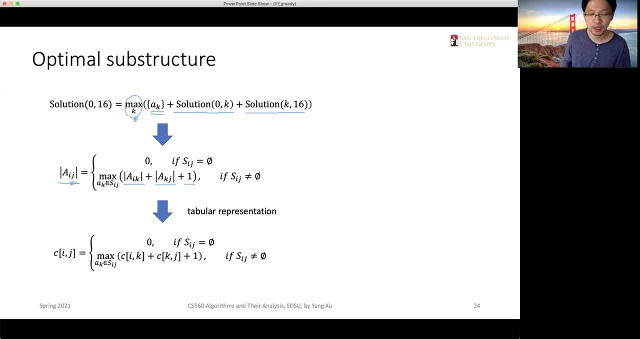 an aj. okay, so if we're gonna solve this use dynamic programming, we're gonna replace this aj with some two uh 2d areas. right, we use aj as the indices for for an element in the 2d area. so we can replace those notations with this: c of ij, c of ik, c of kj plus one and so on. okay, so it's. 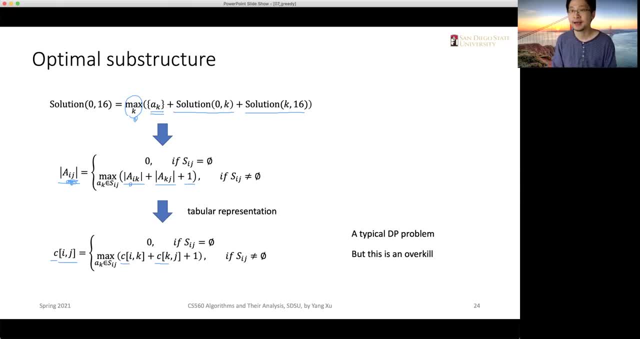 actually a typical dynamic programming, but, uh, this is good. well, i mean, this is correct. right, but this is not necessary. this is an overkill, um, because the special nature of this problem. we don't actually look into all possible sub problems and we just um use a simple heuristic. would be sufficient to, to to solve the problem. okay. 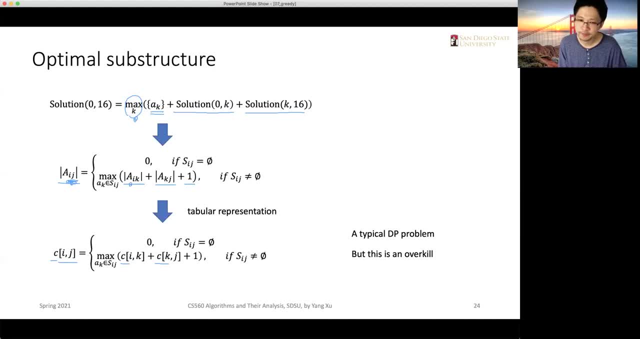 so so i mean, uh, as to the question of how do we decide whether, uh, dynamic programming is an overkill or not, um, i mean, it's a difficult question. i mean, basically, excuse me, how we decide is, uh, is a very, um, um, empirical process. like we, we need to know the. 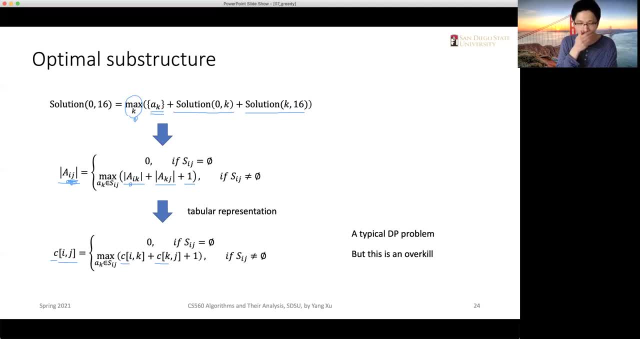 problem. well, we need to know the, excuse me, we need to know the nature of the problem, like in in the case of activity selection. uh, the simple heuristics, like we, we must uh uh select the problem that has the earliest finishing time or latest starting time, would be sufficient to to solve the problem okay. 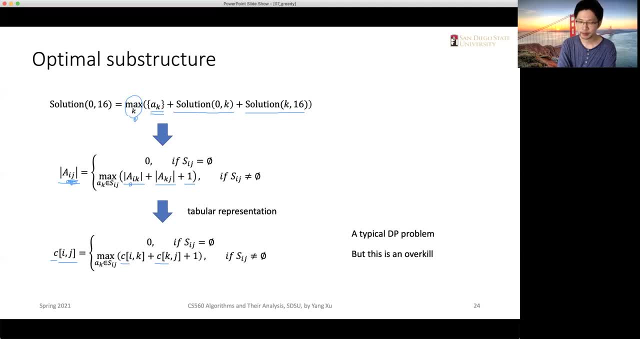 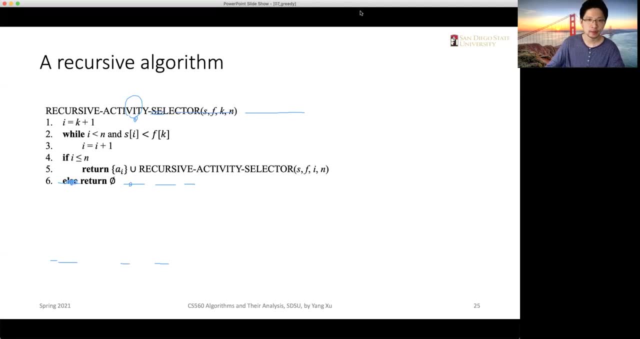 uh really depends on the, depends on the problem. okay, so i mean it's a very simple heuristic, but it's a very simple hayes more. all right. so i think today we can finish the the rest part of uh activity selection. all right. so i think today we can finish the. 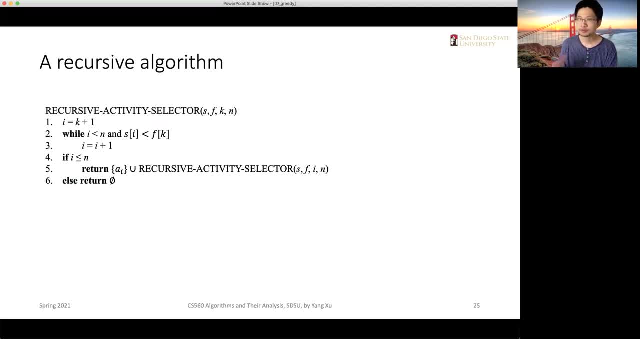 which is a recursive algorithm. which is a recursive algorithm? okay, because we first uh大x, okay because we first uh, okay because we first uh implemented a iterative algorithm. so this recursive algorithm, it's actually uh, uh, it's actually uh reflects. it has- i'm going to OR. 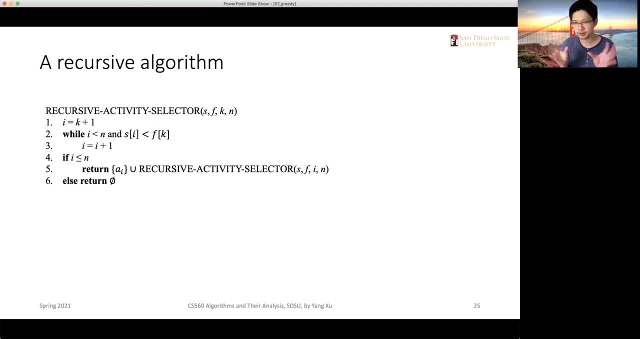 some of this set the way of think of the activities as a set. okay, So there's a union symbol, union operator used in this. Okay, so let's look at the procedure And first of all, it takes some additional inputs. okay, because it's a recursive algorithm, we need to 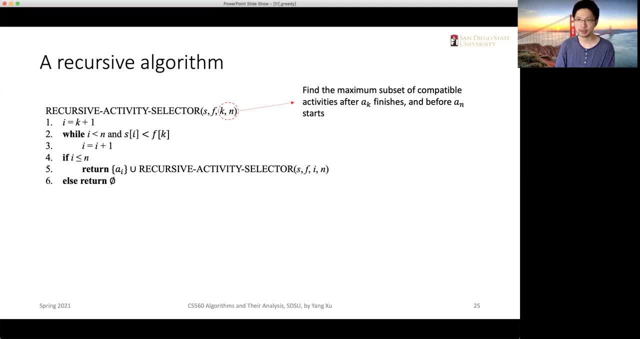 use this additional parameter to indicate whether it's an original problem or a sub-problem. Okay, so this k and n means that we want to find the maximum subset of compatible activities, which is the range of the sub-problem which is after a k finishes and before a n starts. 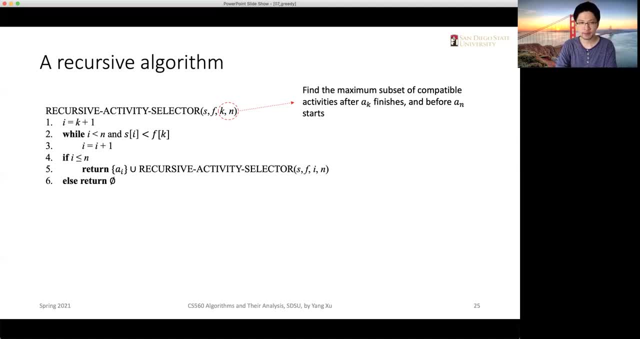 right, That is how we define the range of the sub-problem, And then we will- let's i be the k plus one, because that will be the first one to start right- And we will let aj will use a while loop to iterate. i So this: i will only be incremented if 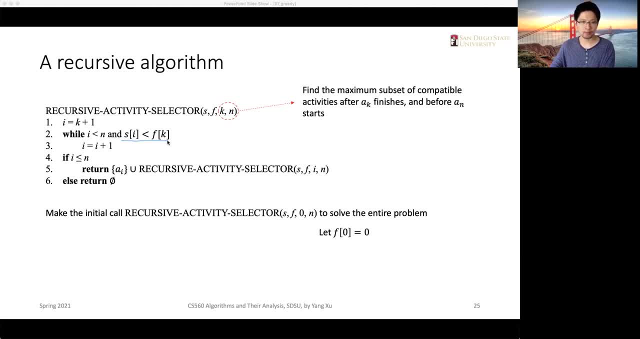 the starting time is earlier than the finishing time. If the starting time of i is earlier than the finishing time, then we will skip that activity. right, We'll skip the activity by increasing, by incrementing i by one, okay, And then, after the while loop is terminated, then we will to give the initial time of the state at the related time before the initially wont one. then print n is counted after that. That's really quite interesting to see This Tibetan method, what various methods go to the significantORs. 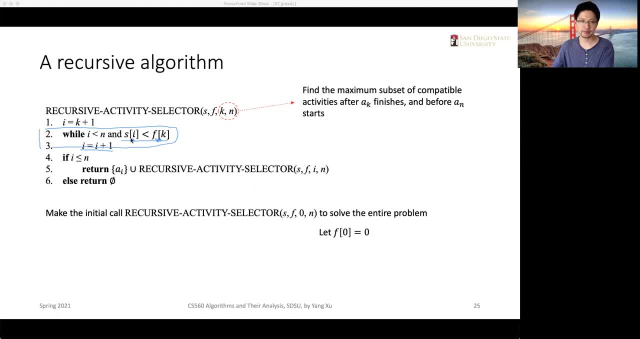 is terminated, which means we find some activity s that has later finishing time than f of k, then if that activity is still within the range, then we will put that activity into the results right, and we call. we will run a recursive call again onto the remainder parts. 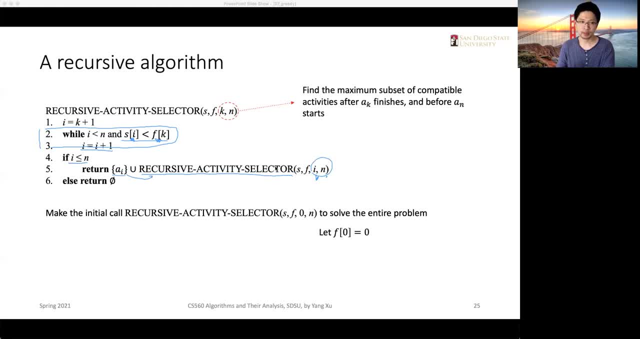 which is from i to n. okay, because now i is selected, we will look at whether we will need to solve the remainder parts. okay, so if that i is is outside the range, then we simply return the empty right. and that would be the boundary condition for this recursion, because when i 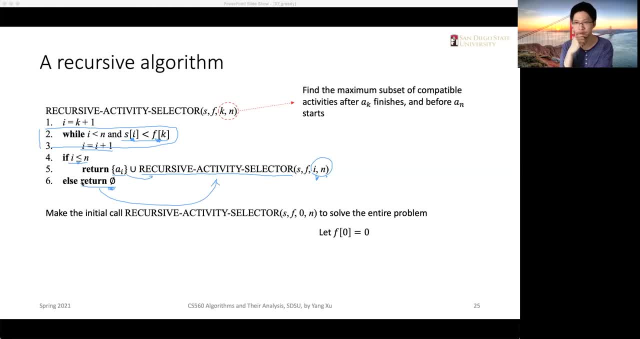 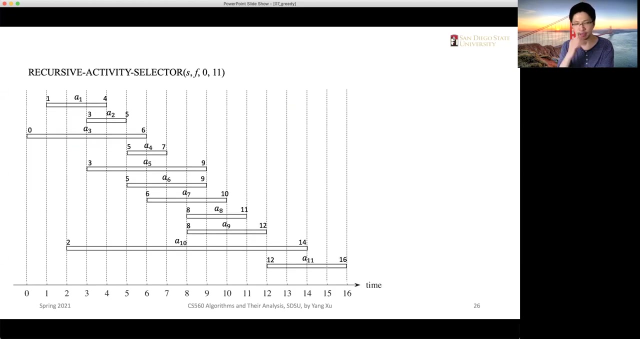 is out of the range, that which means there's no, no, no, no activities can be selected in the remainder parts. so we can quickly look at how this algorithm runs, because our initial condition is that in this case we are solving the entire problem. so we need to let k to be zero and we will let f- zero to be zero. okay, and 11 would be the, the, the. 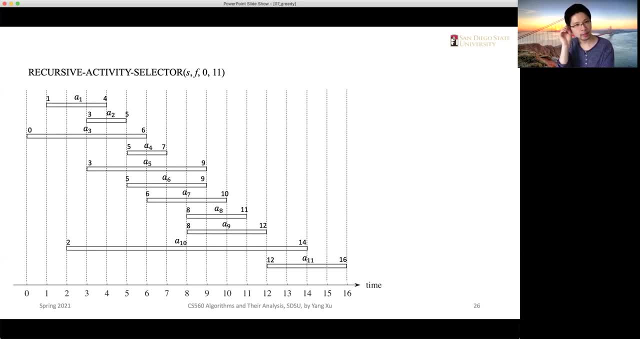 the boundary condition. so we will call the recursive algorithm on between the remainder parts of the range and we will call the recursive algorithm on between the remainder parts of the range and we will call the recursive algorithm on between zero and 11 as an initial call. okay, so look at the body of the this recursive algorithm. 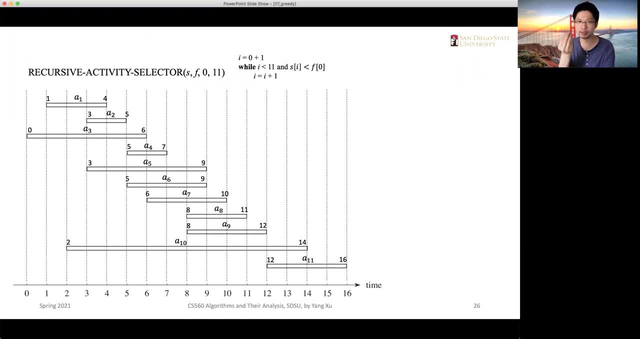 we will let i be start from one right and the i will keep increasing until it finds an activity that has a later finish, a later starting time than f of zero. okay, so when a1 is selected, a1 would be the first. uh, second will be the first active being selected, right, so the next one we? 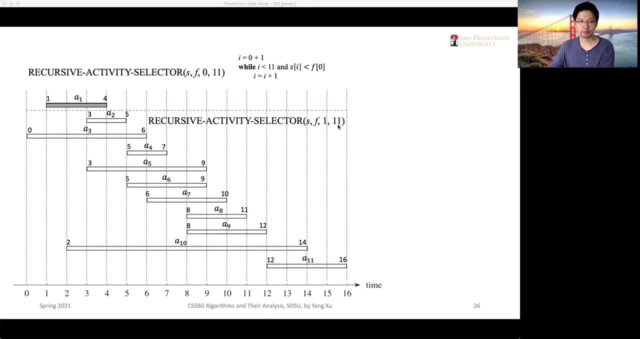 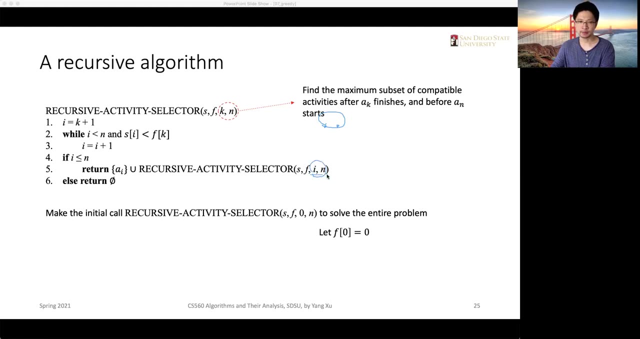 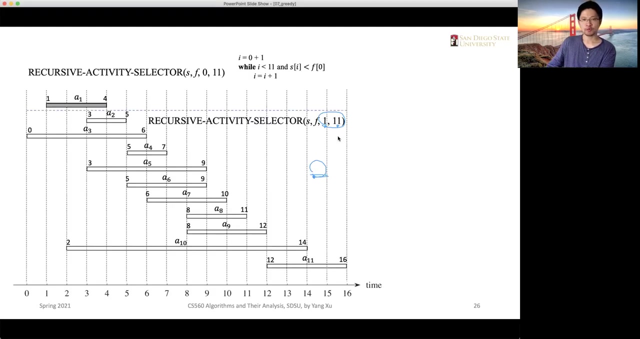 will call a: this recursive algorithm on one, two, from one to eleven, right, remember, within the body of the function, we will let the function uh call the recursive. well, we will make the recursive call between i and n. right, the next recursive call will start from i, right, so the next one will be from one to eleven, right. so, within this recursive call, we will let 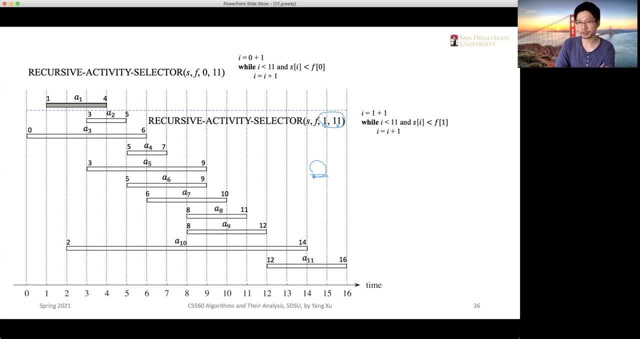 we have the same code executed, but i will start from two right and we will keep increasing until we find a problem that has compatible. that is the first one that has compatible starting time, which is a4 here. okay, so the four will be the new uh condition. 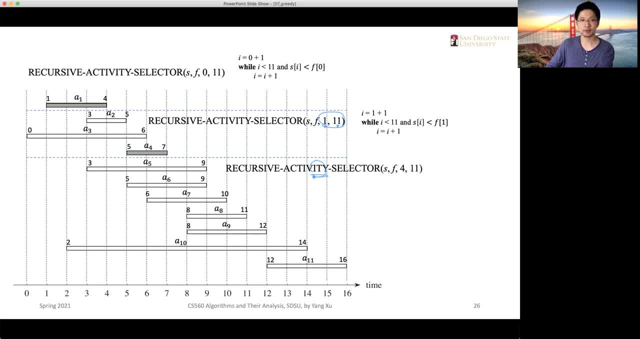 new bound, new starting condition for the recursive call, which is from four to eleven. okay, and then same thing need to be executed within this recursive call. a1, a8 will be selected and then the last one would be from a. the last recursive call would be from a. 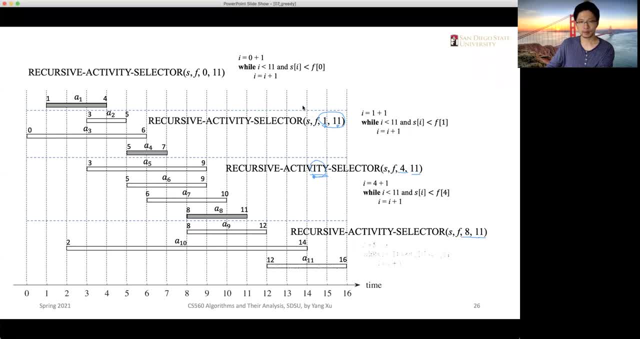 8 to 11.. all right, and the last activity being selected is a11. so after the last recursive call is returned, actually within the body of this recursive call, there is a one more recursive call, um, that is on a11. that is, that has argument sf 11: 11 right. 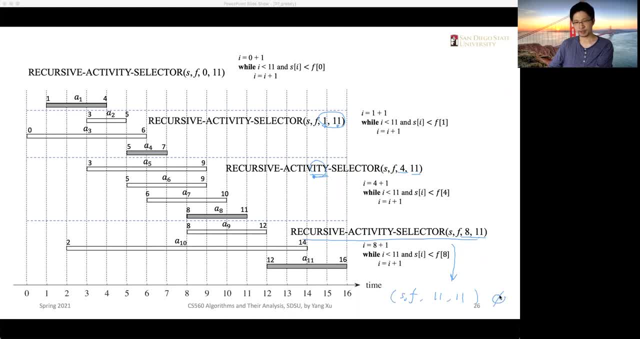 but that will return an empty sets. right, the empty sets will be returned and then we all the recursive calls will be uh returned and the the complete sets of a1, a4, a8 and a11 will be returned. okay, yeah, that is uh how the um recursive algorithm is uh can be defined in this case. 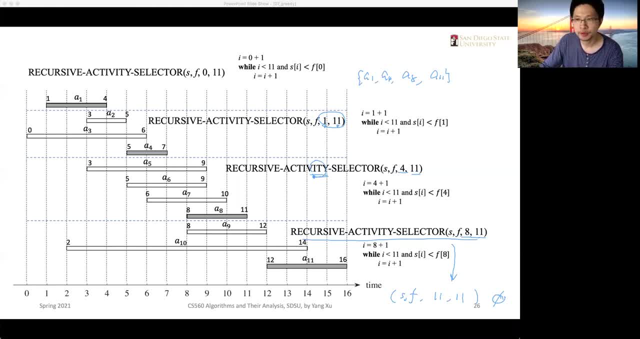 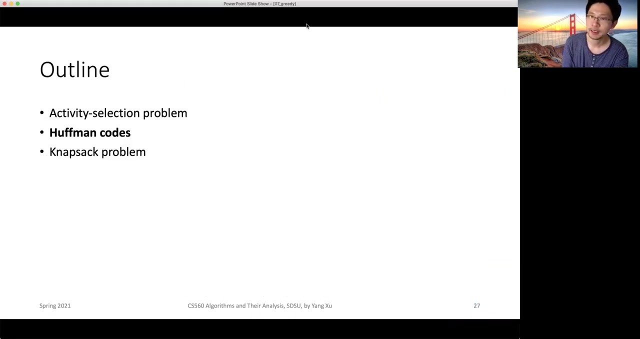 all right. um, i hope you have a good sense of uh what a recursive, uh, what uh an activity selection and uh problem can be solved by this greedy algorithms. in this lecture and on the next thursday's class, we're going to talk about the hoffman codes, which is another, uh typical example of greedy algorithm making really choices. 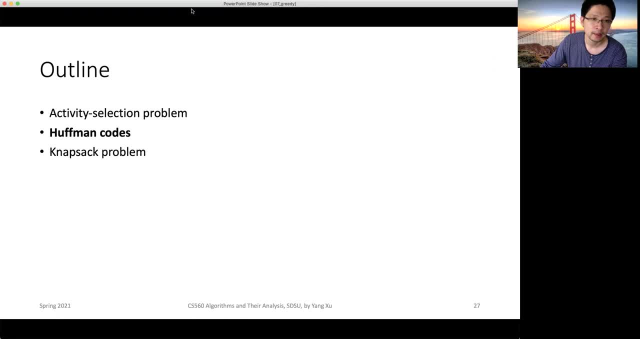 at each step of an of an algorithm, and also we'll talk about, uh, knapsack problem. so it's knapsack is a very classical example that connects with both dynamic programming. okay, and a variance of knapsack is actually only solvable with dynamic programming, while